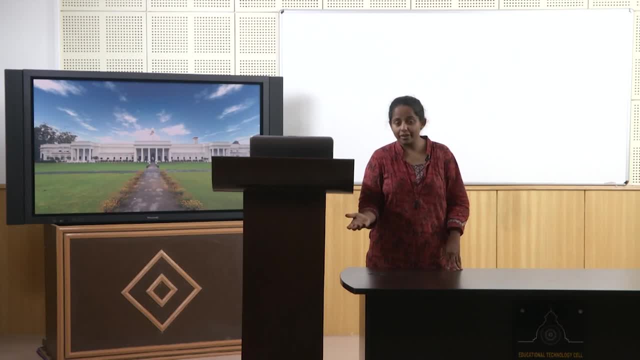 a group of heterotrophs who simply degrade the organics. But when science developed further, we understood that there is not just one kind of microbe or microorganism that is at work. So what used to be collectively referred to as biomass when we talked about sludge- 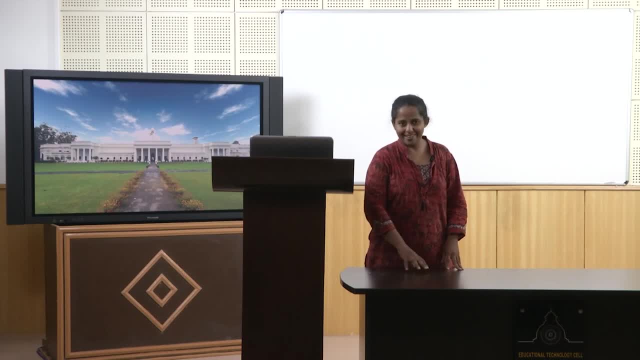 now started being respected in a way and distinguished in sense that now we had heterotrophic bacteria, autotrophic bacteria, we had anoxic and anoxic microorganisms and this is how we started respecting that not all microbes are similar As the science of microbiology. 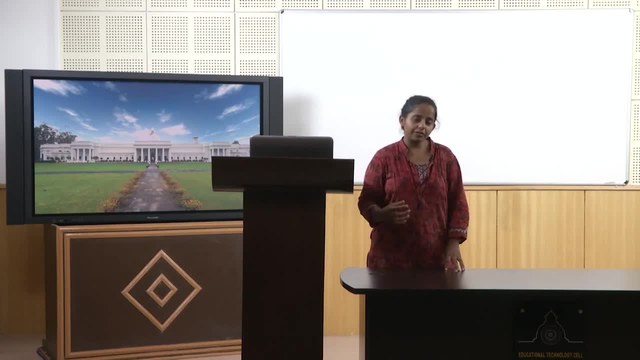 developed even further. we understood that even within these broad classifications, such as heterotrophic microbes, there are there is a huge diversity. there are many different kinds of microbes. In past two decades, past three decades now, microbiology has given us techniques such as genetic sequencing, where we can actually sequence the genome and the genes of 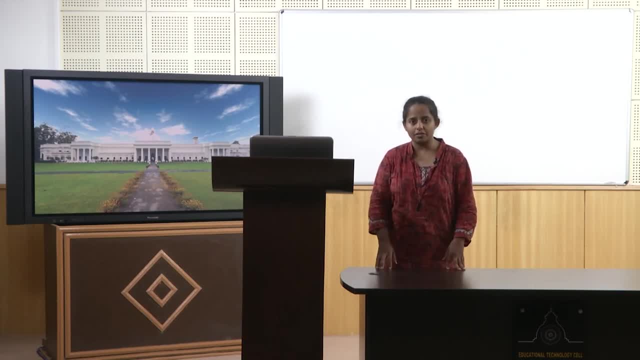 bacteria and understand how similar or how far apart they are from each other. And with onset and discovery of these wonderful techniques, what we have now is a much broader and more clear vision of applied environmental microbiology. Unfortunately, in many regions of the world, India included, the microbiology of environment and its applications are not really well understood and 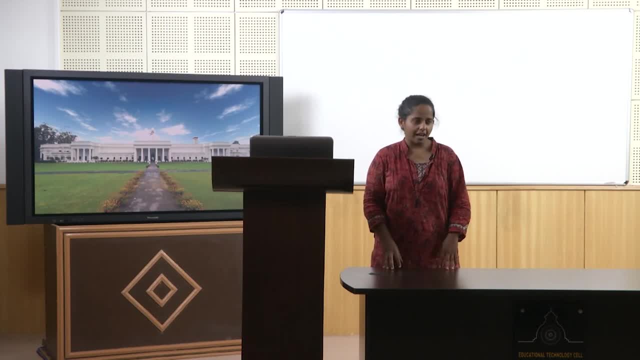 mostly confined to the domain of pure research and is ascribed as something that perhaps a biotechnician would do or somebody with a biological background would do. And this is where I want to give you a small introduction that you do not have to be familiar with biology, let alone. 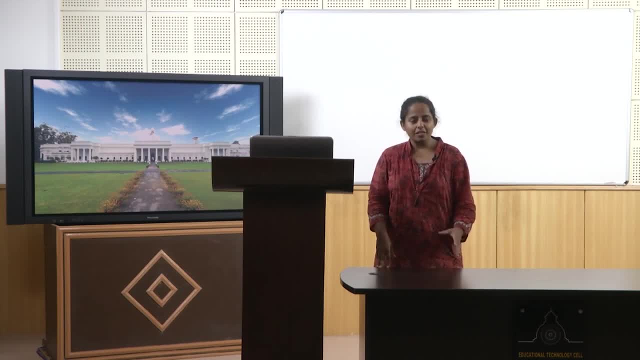 microbiology in order to understand this course really well. What is important in this course for you, from you, is that you pay attention to what is taught and covered in the lectures and honestly, sincerely, do the assignment Now. today being the first lecture, I would like to take some time to make you more familiar with 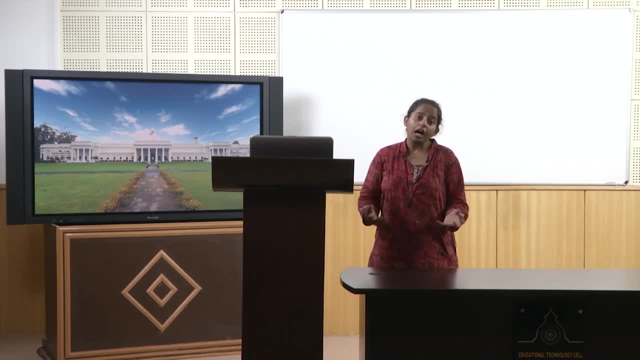 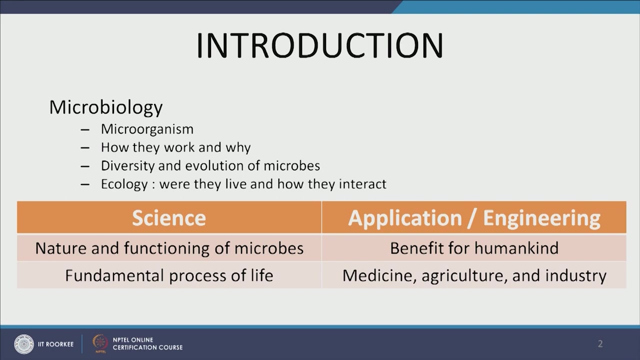 what we are going to discover together in this course and how it might be applicable for you. Now, in microbiology in general, we talk about microorganisms. we want to know who they are, and this is where microbiology and biology get very tricky and put off many engineers and scientists and science students, because there is a perception in 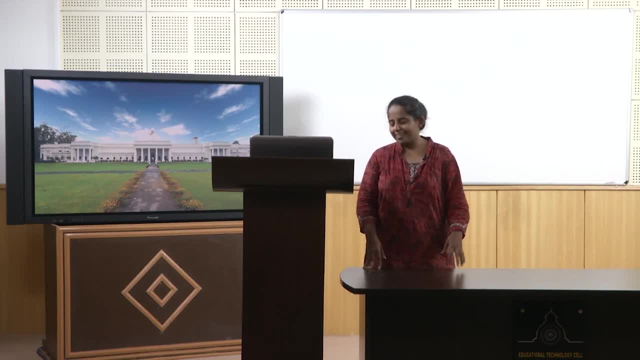 microbiology. we need to memorize so many things by rote and I assure you in this course you do not need to memorize different names, you don't need to know how chronoarchivata is different from you archivata, but you do need to understand how the microbiology in itself works and if you 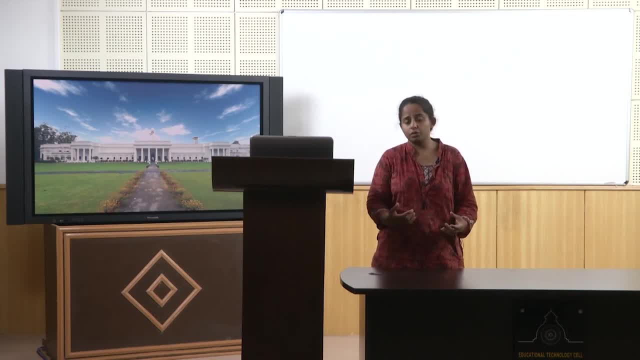 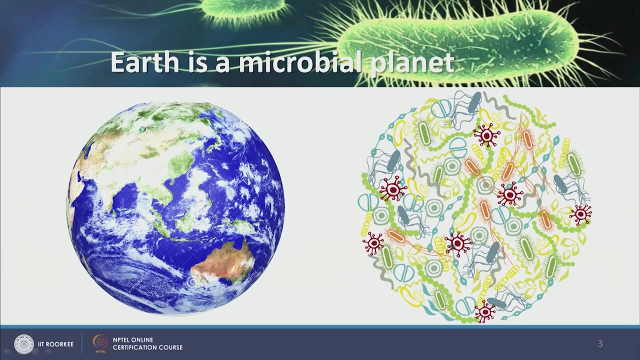 what information do you need in order to understand why microbes are doing what they're doing and, in the first place, how what they're doing and how you can tweak that in order to serve your environmental purposes? which brings us to the second bullet here. The first aspect is to understand what microorganisms are present. 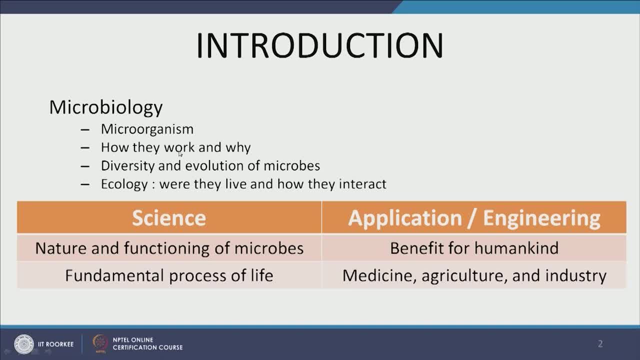 how they work and why they do what they do and what it results in is an understanding of the immense diversity of microbes and how they evolve from one kind of microorganism to another microorganism. and speaking of diversity of microorganisms, it's really beautiful to note that most microbiologists, including myself, believe that we have 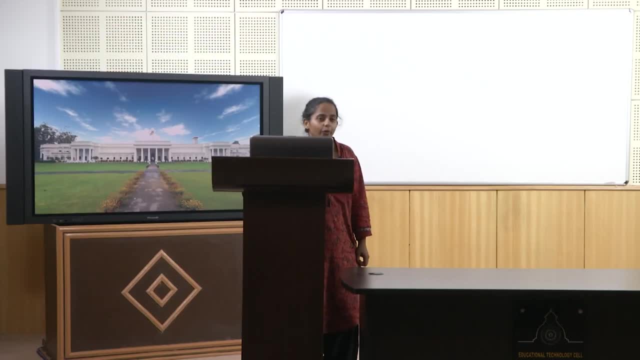 barely scratched the surface. we believe that we know less than one percent of microbes that are there in in our on our earth, and the fourth bullet here talks about ecology, which is, where do they live and how do they interact with each other, and this is particularly important for environmental. 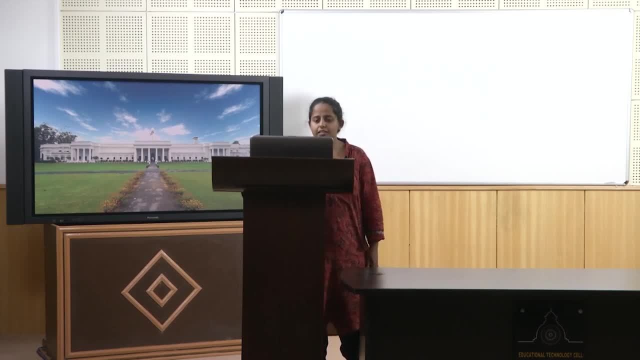 engineers, environmental scientists and technicians. we want to understand how micros behave with each other and how they behave with the environment, how they are influenced by the environment and how do they influence the environment in return. microbiology in itself has two legs on which it stands. one is the scientific aspect and the other is the application on the engineering. 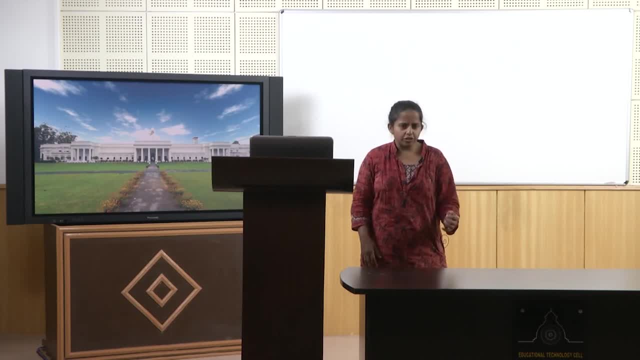 aspect. the science wants to know the nature of microbes, how the microbes function, what's the fundamental process of life, what's the biochemistry of life, whereas the application aspect and the engineering aspect wants to know. okay, how can i use this information that i have to improve our living standard to benefit our humanity? 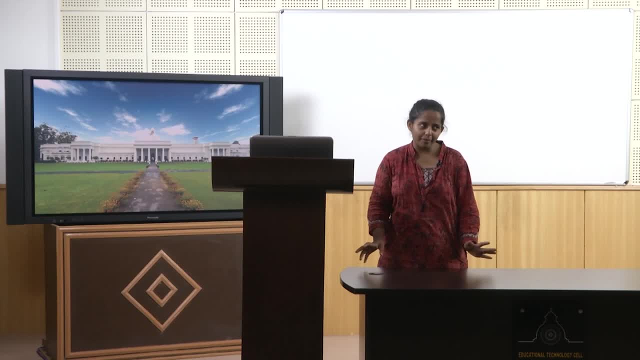 to make our civilizations more sustainable so that we can live happily on the third for longer time. and the application aspect also looks into medicine, engineering and agriculture, and now we have an emerging field of industrial microbiology, and lot of what you study in this course will actually help you address any of these applications. in this course, we are not focusing as much on 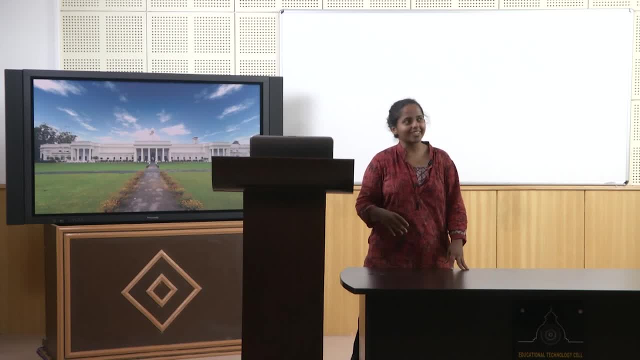 science and that's why you get a good riddance from all those scientific names and techno long enumerations of microbes and you can directly jump into how we can use this information that we have to better our world, to make better medicines, to have cleaner surface water, to have cleaner groundwater. 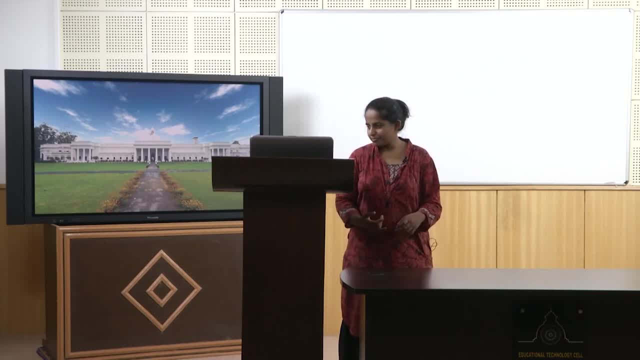 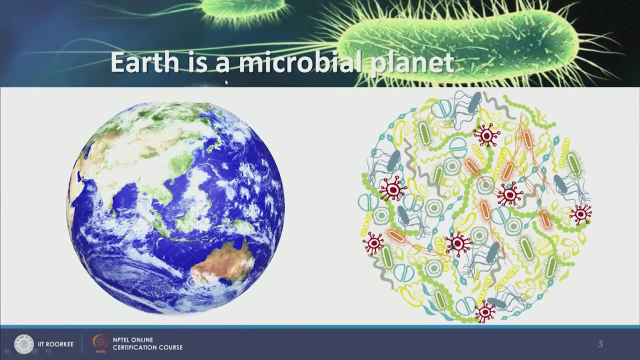 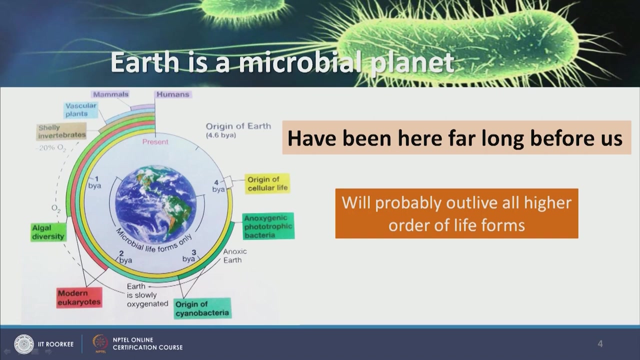 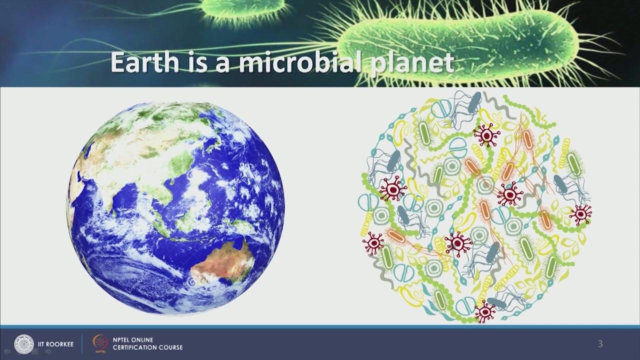 cleaner air now and just how to be healthier now. this is very important to understand that. why applied environmental microbiology is very relevant today. we think of earth in terms of lithosphere and in terms of lithosphere, it has lot of blue in it. so all the maps, so there's lot of water and 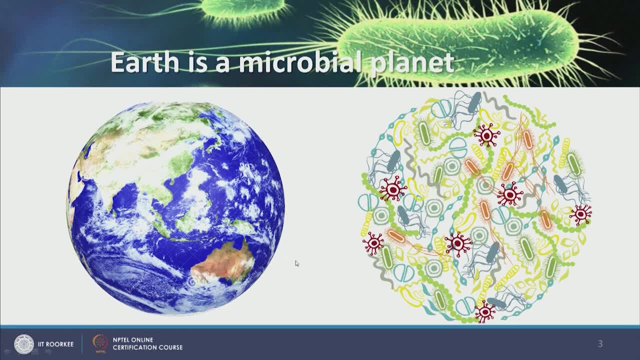 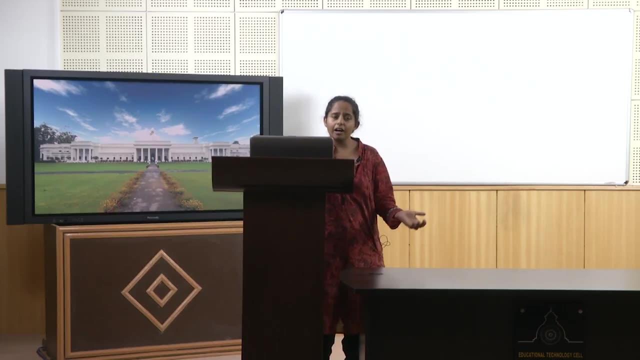 then there is land. what is hiding in this picture are the tons of microbes that actually inhabit the earth, and if we look at, from biomass perspective, the percentage of carbon that is stored in microbes, we can say that the life on earth is mostly in microbial form, not in the higher forms. 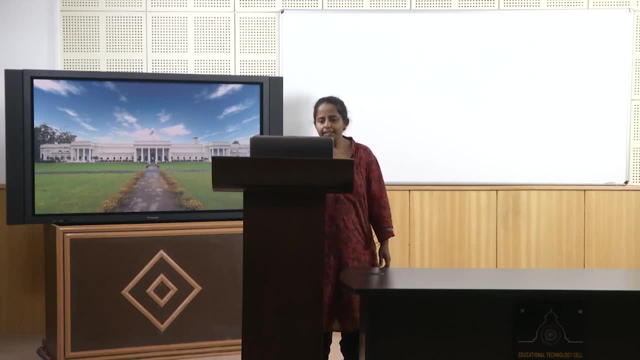 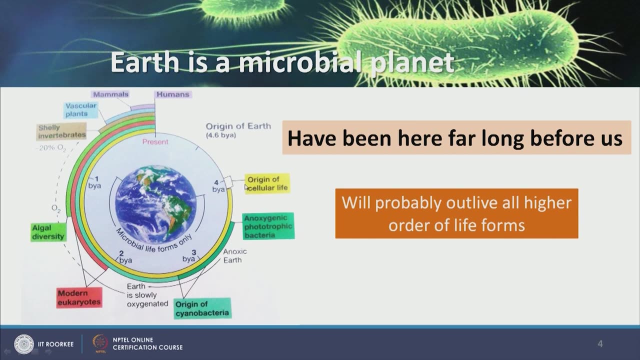 of life that we see and let's look at the origin of life, origin of earth, and this will cement further our understanding that earth is a microbial planet. It is said that earth is nearly 4.6 billion years old and the life started some 4 billion. 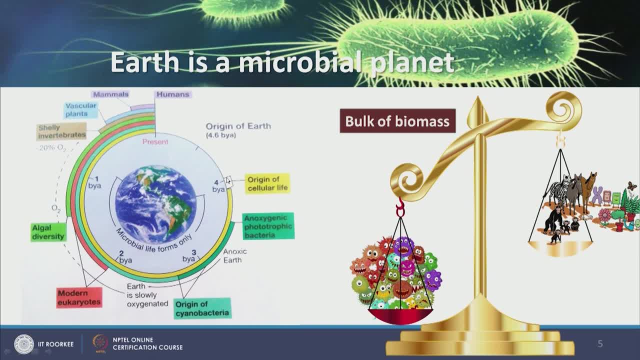 years ago. that is origin of cellular life. ok, Now we are understanding that non cellular forms of life started way before 4 billion years, but definitely the cellular life started 4 billion years. that is where the microbes came, And then somewhere between 4 and 3 billion years we got anoxic phototrophic bacteria. 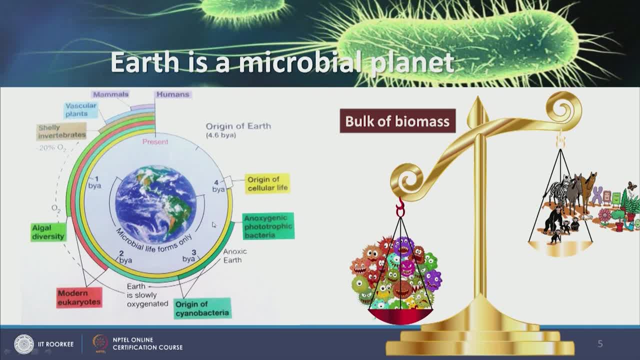 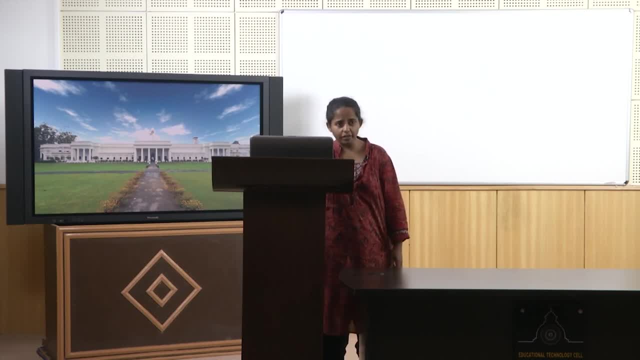 and this is very beautiful to understand At this time. for all these billions of years, earth was anoxic, which is another way of saying there was no oxygen on earth. earth was an anaerobic environment and humans, as now we are, could not have existed, survived at all in this, on this earth, then 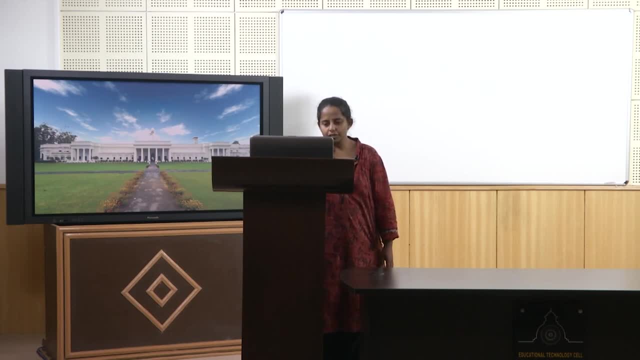 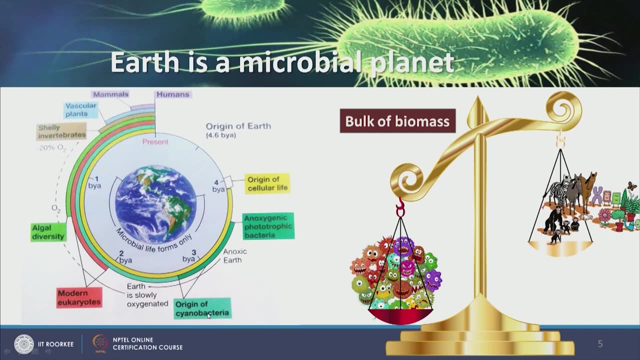 However, a miracle started happening sometime around 3 billion years When, Between 3 billions and 2 billion years ago, cyanobacteria- a green, beautiful bacteria- beautiful under microscope, by the way- green cyanobacteria- came over, evolved on earth. and what this cyanobacteria? 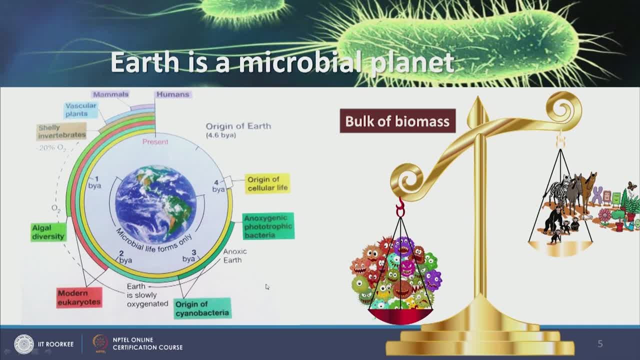 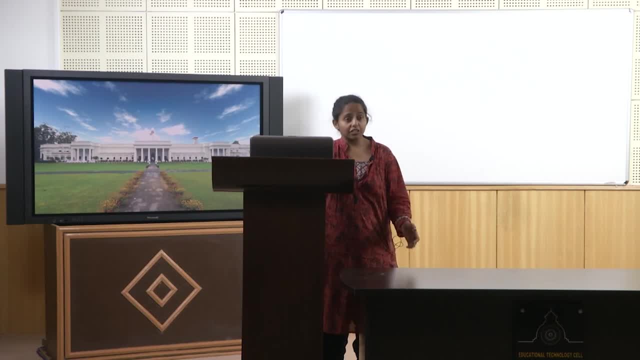 started doing is started using the light to produce food, which is something we are familiar with as photosynthesis in case of plants, and started generating oxygen. So, over the course of Next billion years, the earth was slowly oxygenated. So from this primitive form of life- and we are using primitive in sense of time, not necessarily- in sense of complexity? definitely not in sense of complexity, I want to be clear. but in terms of time, the life started also incorporating and exploring the aerobic forms of existence. So around 2 billion years ago, modern eukaryotes- now- this is a technical term- eukaryote prokaryotes. 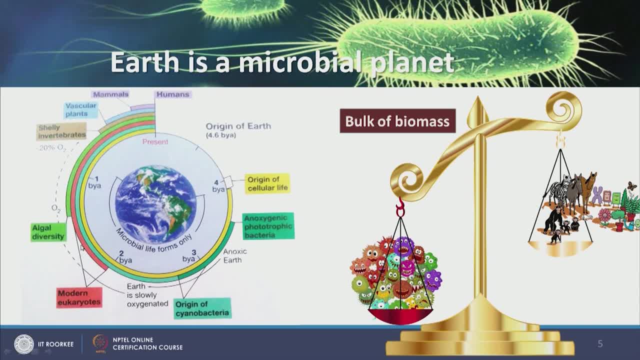 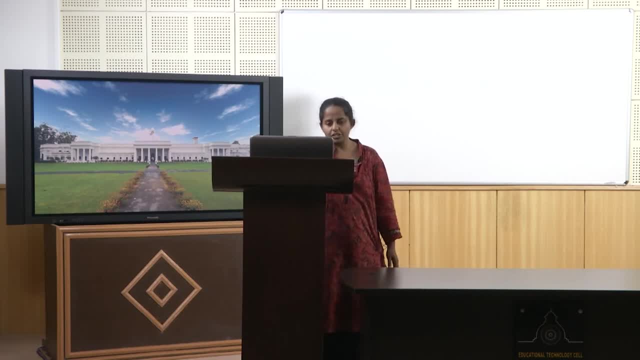 u means true, karyon means nucleus, So something that has a particular kind of cell which we call as eukaryotes. and it might be helpful to mention that humans are eukaryotes. all the higher order of life have eukaryotic. 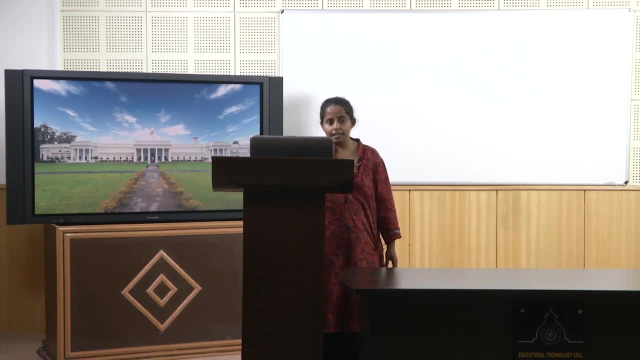 cell, and the uniqueness with eukaryotic cell, as we will see later, is that they have a nuclear membrane in which they have destroyed the genetic material. So some 2 billion years ago, these higher forms of life, the modern eukaryotes, came into picture. 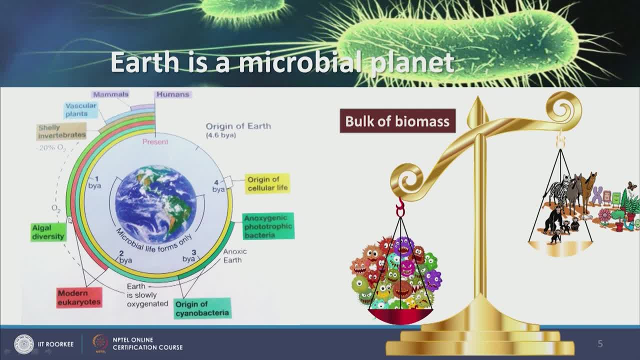 and then, low and behold, very soon we had algae, we had this photosynthetic eukaryotic organisms and then much, actually much near the present. some 500 million years ago, Shelly invertebrates came, vascular plants, mammals and humans are relatively recent. 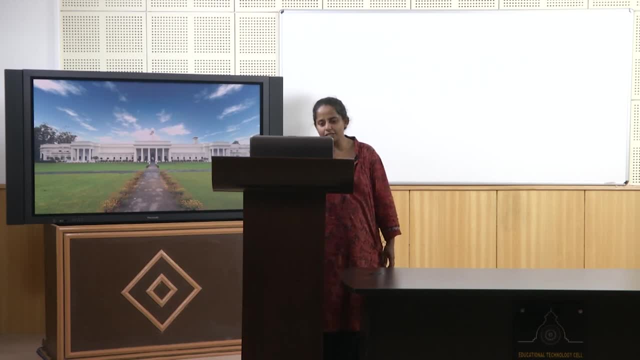 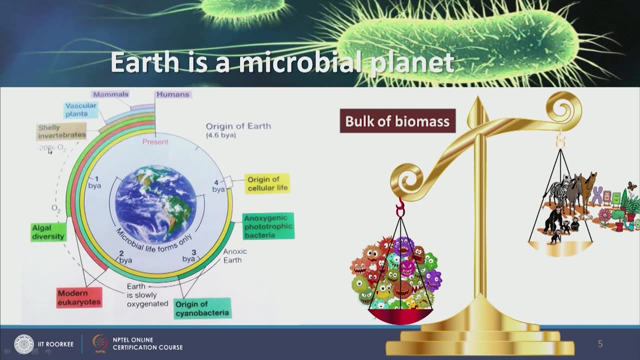 phenomena, very recent phenomena. So we can see, for nearly 4.6 billion years of earths existence, We have At least three and half years of only microbial existence and if we look at in terms of biomass, more organic carbon is stored in microbes than in all higher forms of life combined. 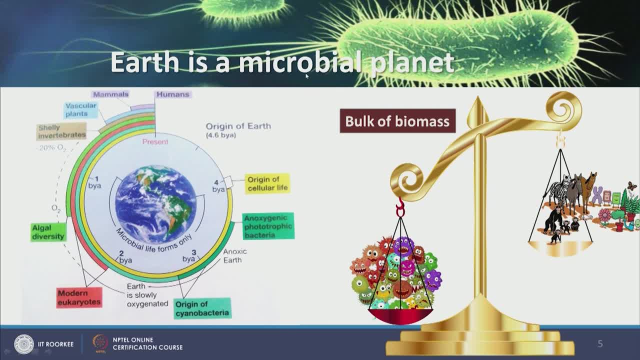 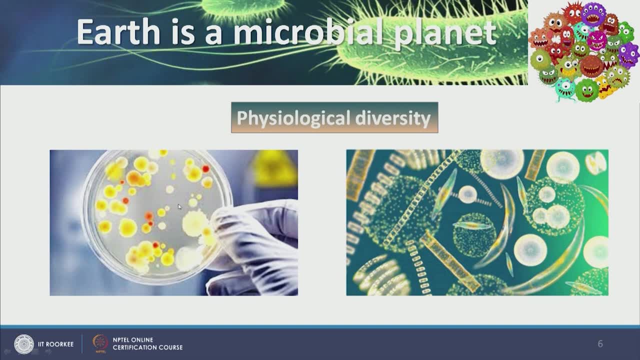 and thus we are assured, as microbiologist, that earth is a microbial planet. Now in this, in this slide, we have two beautiful pictures. on left, we have a scientist showing off a plate with different microbes growing. Now in this plate, it is very beautiful to know that each of these colonies have emerged. 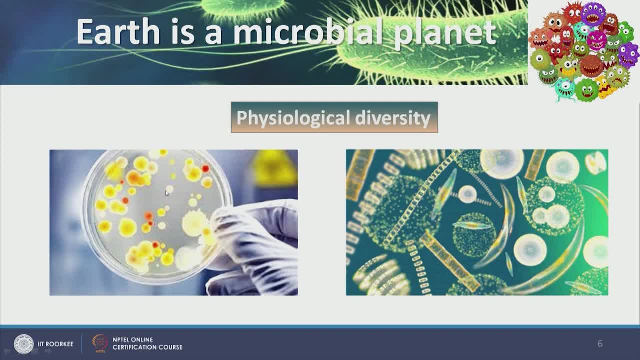 from a single bacterial cell. these are bacterial colonies, by the way, and on the right side we have a picture- and this is an artist's impression- of three dimensional picture of microbes of different morphologies, different shapes. So, if you look at this visually, on the left in our plate we have 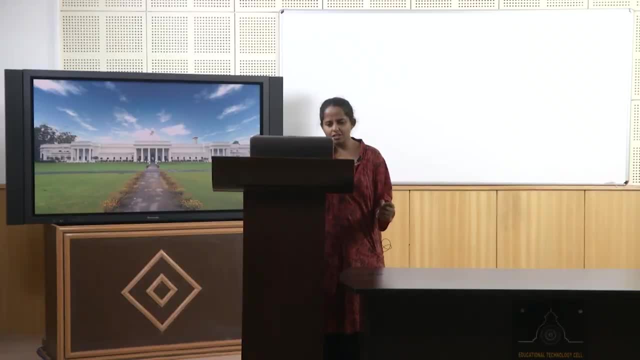 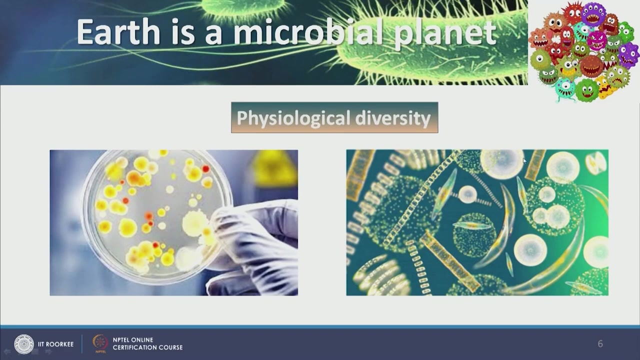 Microbes that look very similar. the colonies that they make are somewhat circular and start with red and as they spread out they get more yellow and then even white. On the right side we have these beautiful, strange and very distinct geometries. some of them are caucus shape or round shape. some of them are rod shape. some of them look like 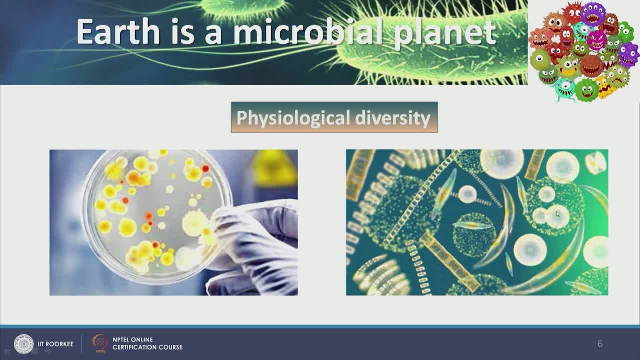 these galaxies, and some of them look like dots that are clustered together, and what this wants to highlight is that, on a physiological level, There is immense diversity in nature, as represented by the right picture, and what we humans have been able to capture in lab is a small fraction, only one kind of microbe, and that is the reasoning. 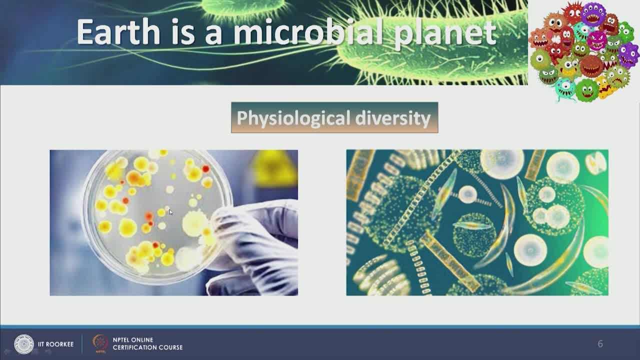 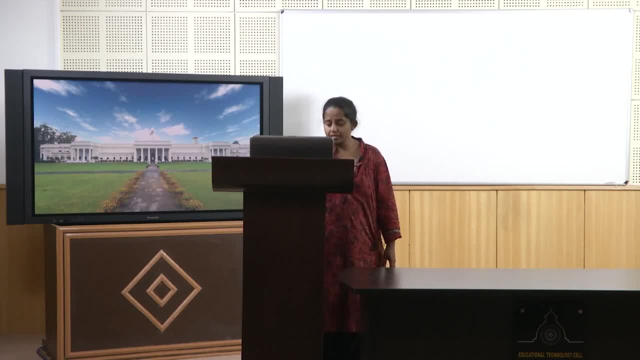 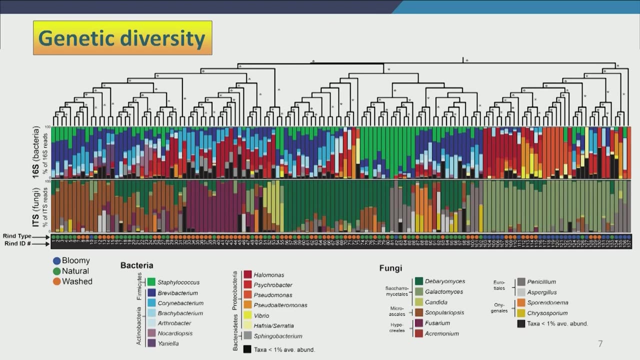 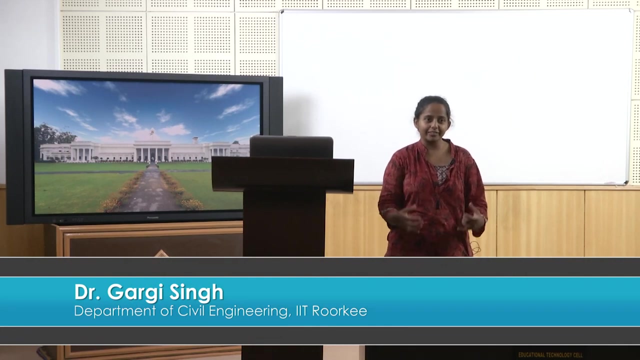 behind the popular saying that we have only scratched the surface of environmental microbiology. This is in terms of physiology. so this is how microbes look. Now what microbes are beneath their looks is even more complicated and more interesting. So in higher order of life, we see two mammals who have, who stand upright on two legs with 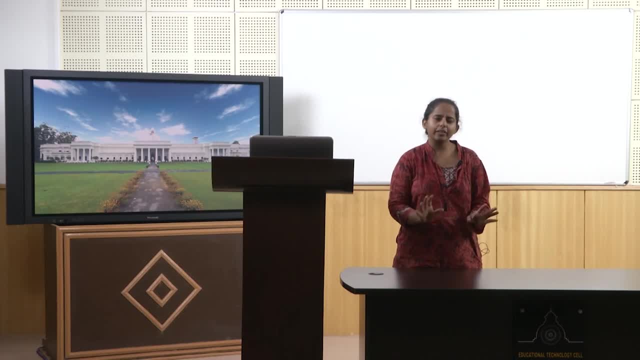 two hands and upright body and a head, and we assume, okay, they are humans, they must be similar to each other, and we do know that, genetically, the humans are very similar to each other. In physiology, we are very similar as well. however, in terms of, in case of microbes, we 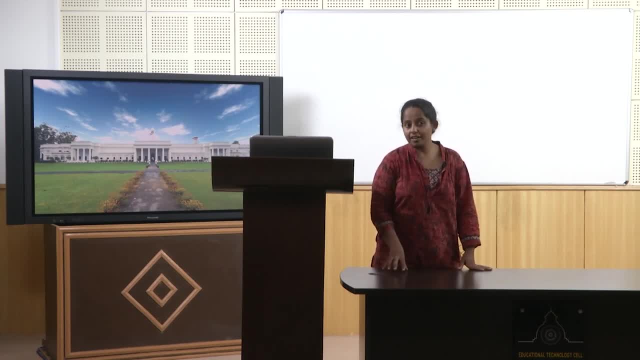 cannot have similar. similar ideology doesn't work for microbes. Two microbes that are perfectly spherical and maybe give response similarly to different light that we throw on them might be very distinct and very unique in their behavior. for example, Ecoli: two strains of Ecoli have exactly similar morphology. one might be benign. 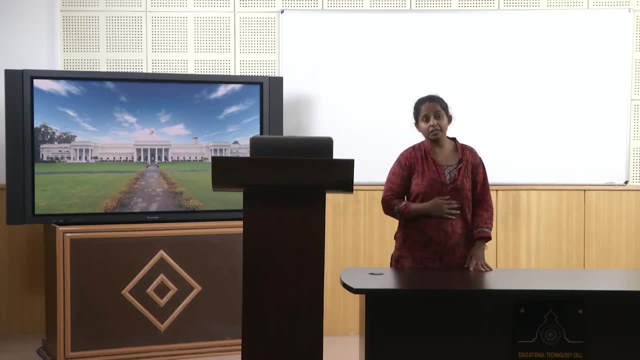 and might actually help when it is in my gut, the other might kill me in couple of hours. so same strain, same species of microbes that look very similar, have similar morphologies, might be very different in their activity. and let us say, even if they are similar in their activity, they might be very, very different. 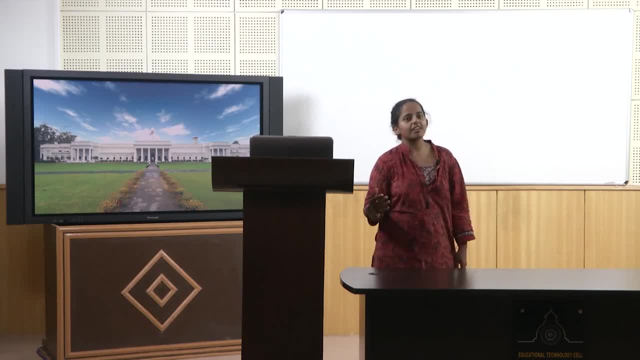 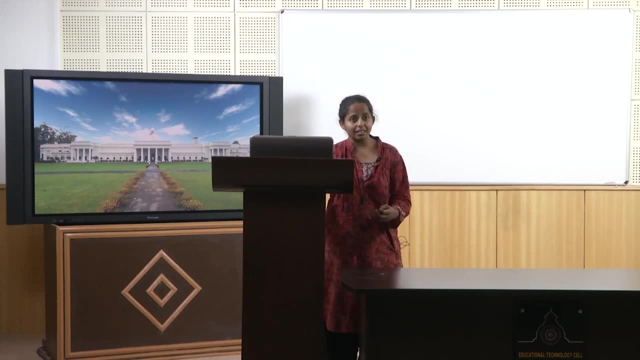 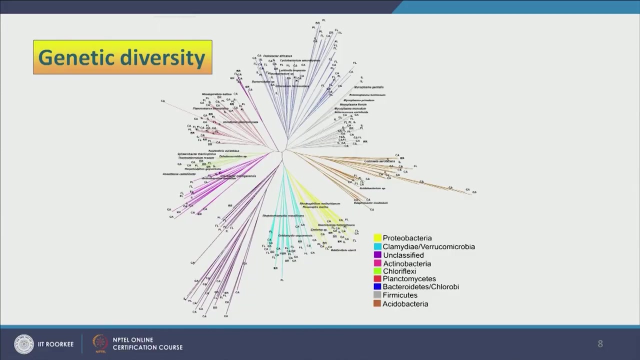 in their genetics. so we will get through what these genes are, what the genetics are is, but for now just know that genetic diversity tells me the essential differences that are there in the makeup, in the code of life in these microbes. so in here you have a dendrogram which has been represented in a tree of life. 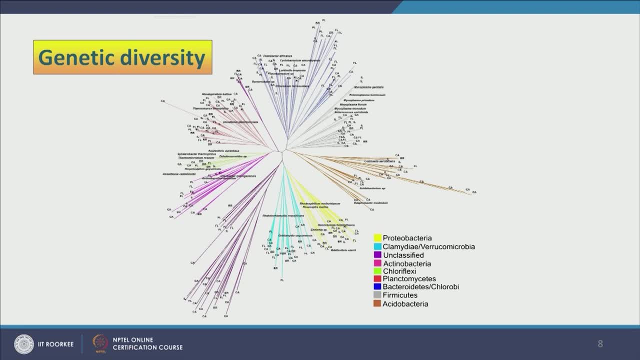 form, This dendrogram format showing each of these streaks represent. each of these streaks represent a particular kind of microbe, a particular very distinct from each other. the closer two microbes are to each other, for example, all the blue ones that have clustered here together. 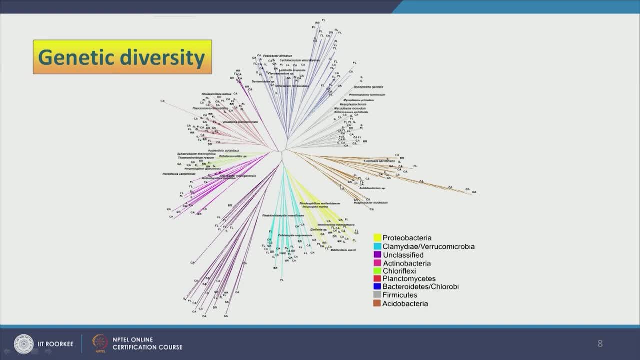 and then the brown ones have clustered, the closer they are to each other. we can say that more similar these microbes are to each other. the color represents the broad phylum that they belong to, and I can speak with good level of accuracy That even though if they are two clustered, two bacteria are clustered closer, for example. 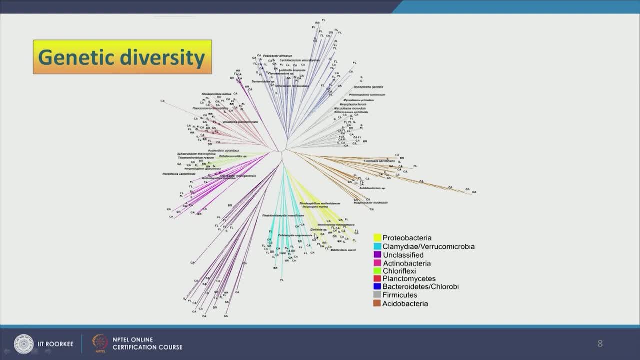 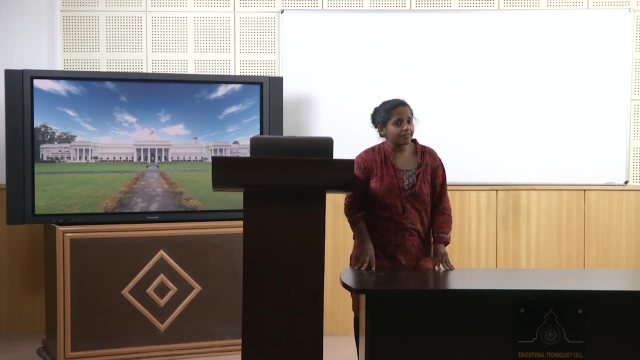 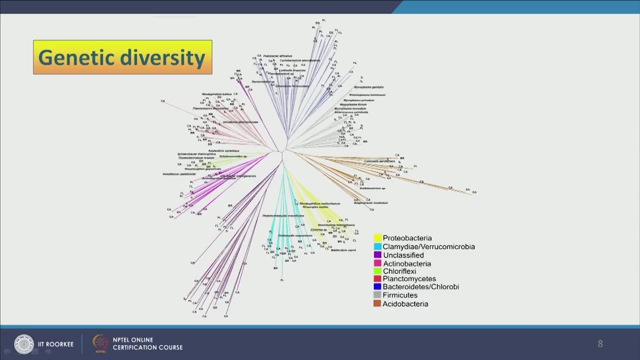 the yellow, or proteobacteria. and even if two lines are very close to each other, we might come under the impression that overall they might behave similarly- yeah, but they might be as different as we are from algae. so in this particular picture here, which says genetic diversity, two lines that are very close to each other and have same color might be very 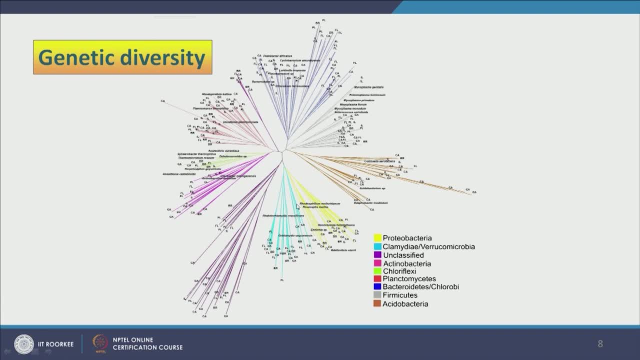 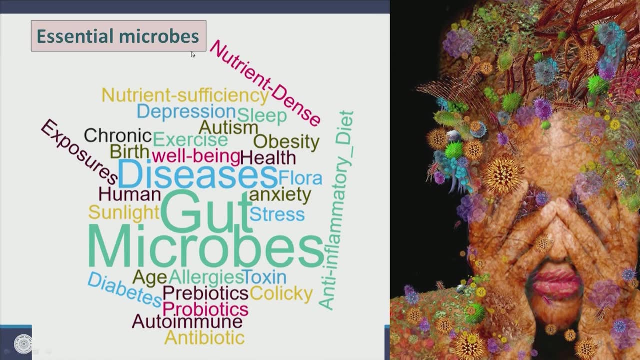 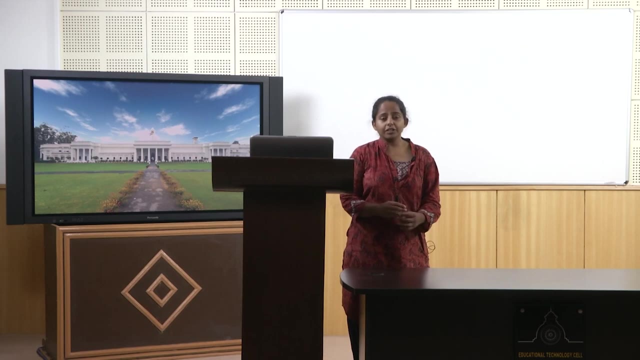 different in their behavior And in their genes. now this slide talks about a very important aspect of essential microbes. why is this important to know? why do I want to know about tree of life? why do I want to know about genetic and physiological diversity? because there are microbes that directly impact. 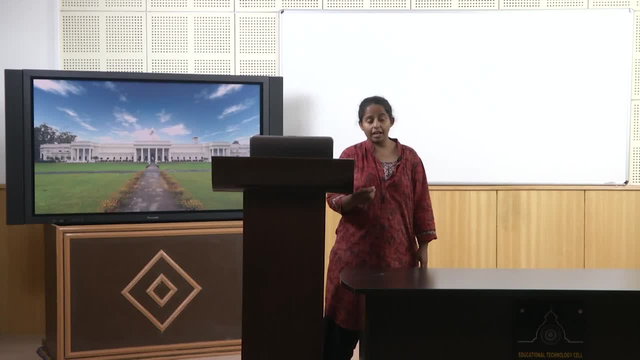 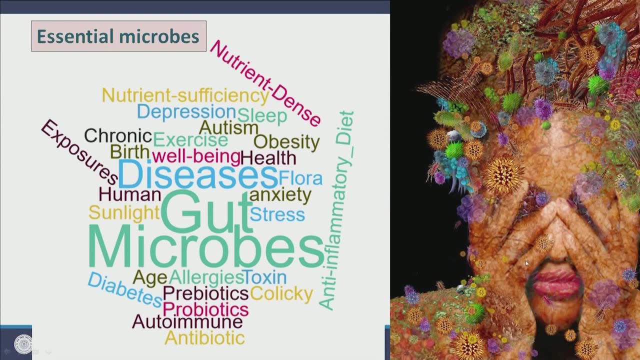 our health that impact our environment, impact our industry, such as agriculture and other industries, and this is on right. there is a picture from, I think, time magazine- this was the cover of that magazine- Showing how- Showing how human beings are inhabited by microbes, and I think this is a great time. 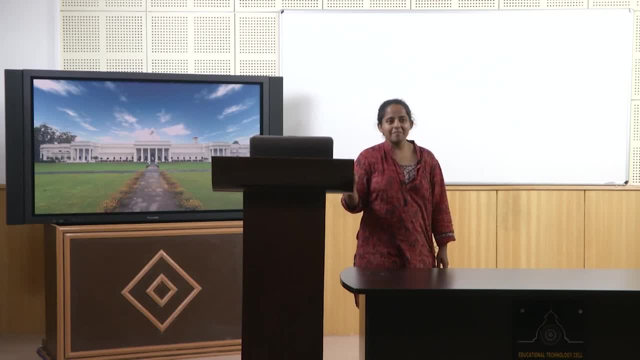 to share this, in case you did not already know that in our human bodies we are a minority, and what this means is, for every single human cell in your body, we have at least ten non human cells, ten microbial cells. So just take a moment to ponder about this: we are a minority in our own body. now are 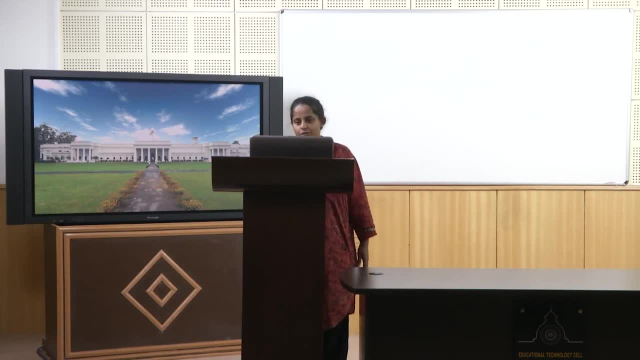 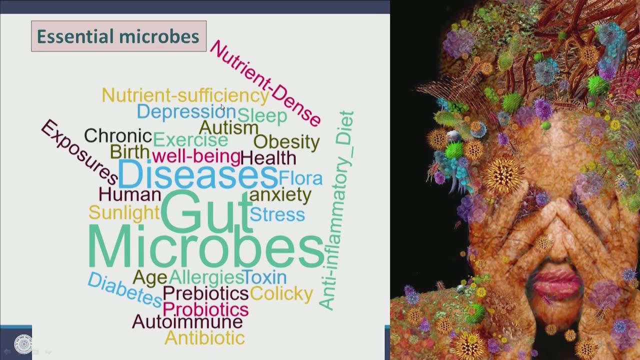 we really humans then, and this is the picture that So So that time use to illustrate this novel finding that we have, and now we know that microbes affect us in terms of nutrition. they actually will allow us, and will see this very soon, that, given the right microbes in the gut, we in the gut we might not never face. 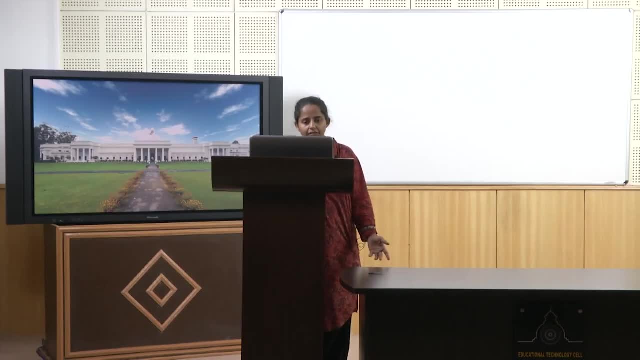 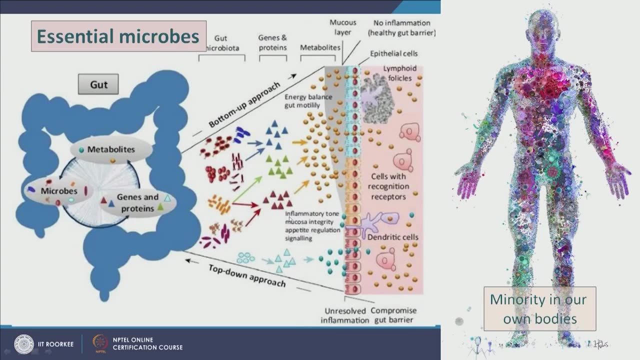 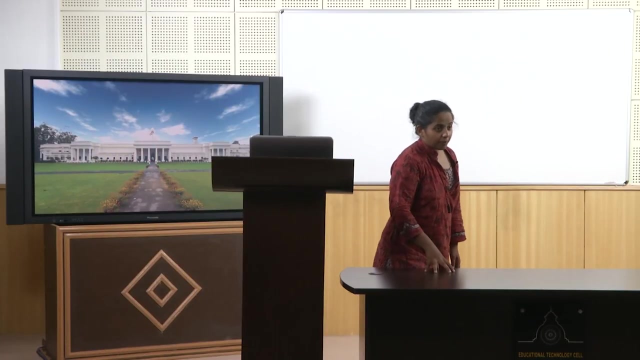 nutrition deficiency or if you do not have those good microbes, you might release our problem. and coming back to the essential microbes, this picture shows some wonderful research that is going on Right Now now to see how microbes impact our health. Now it's a very important thing for you to understand that, even though we talk about 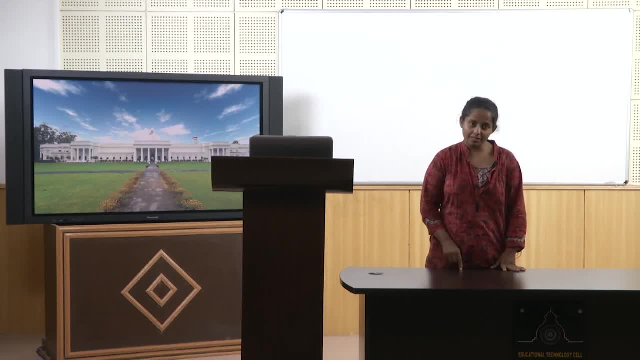 environmental engineering. environment is anything that surrounds us, So we can have at least three different kinds of environment. Broadly speaking, we have an external environment, and then we have an internal environment, And internal environment would include, for example, my gut microbes. 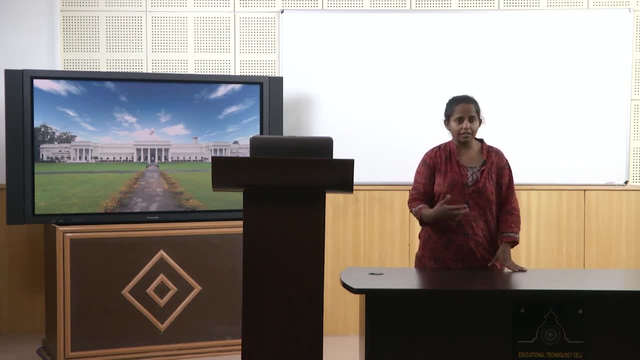 What's going on in my gut. We know that human gut is heavily colonized by bacteria and other microbes And they are essential. Most of them are very important for our health. If we lose them, we fall sick. Then we have microbes in the outer environment which impact things like our climate, which 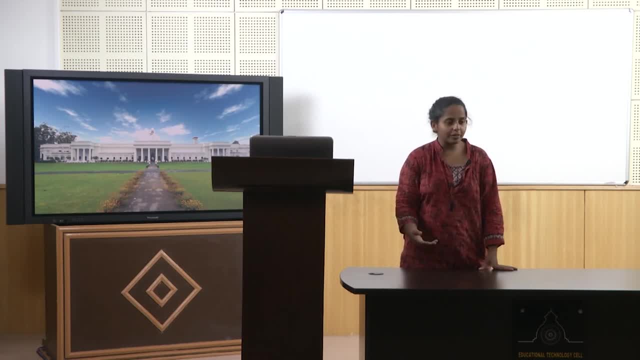 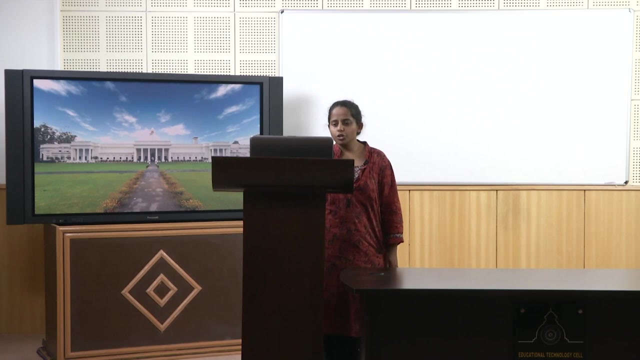 impact how much oxygen goes out in the atmosphere. They influence how our waste degrades, how our landfills behave, how our wastewater treatment will be successful or not, what problems we might face. will our sludge float or not? And the latest research, as represented in this slide, is showing that it's not there. 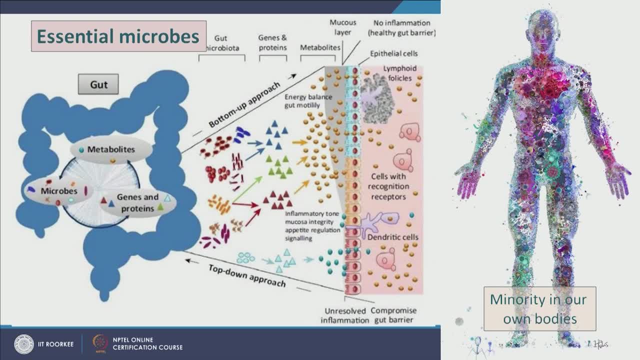 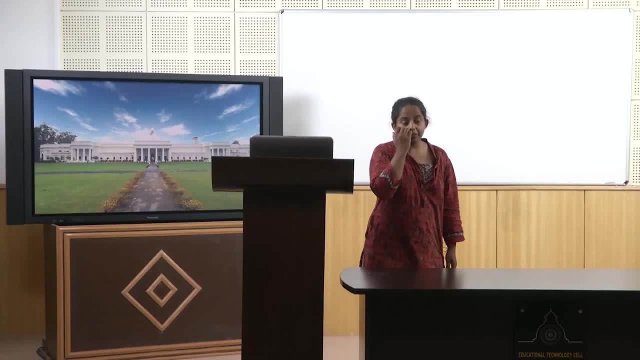 is no clear division between external and internal environment. The external influences the internal and the internal influences the external. Let me give you an example. You are sitting in a room- clean room, like the one I am standing in right now- and a dirty, muddy dog walks in. 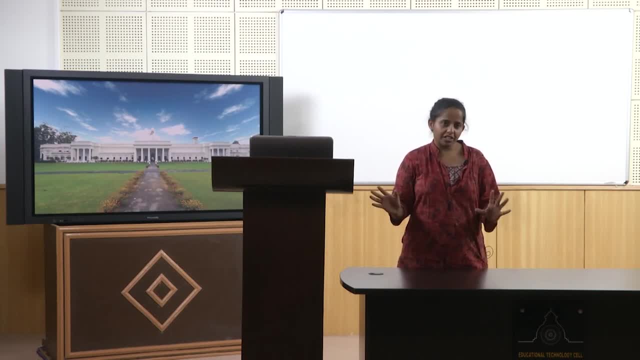 Then the dog, because the dog is wet, let's imagine, and when the dog shakes itself to get rid of the water, He also sprays these micro bio aerosols with lot of microbes in the air. You happen to inhale some of them. 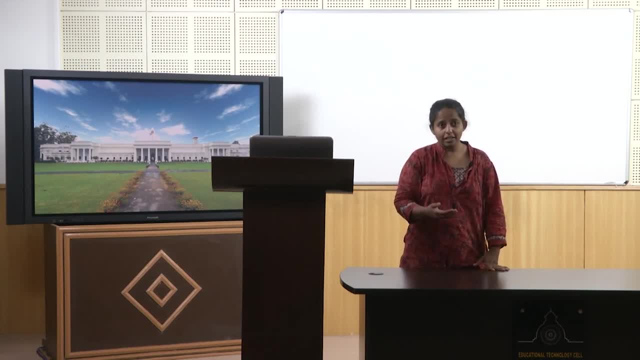 Now, these microbes that are in the air thanks to the dog that walked in will colonize your nose, your nostrils, maybe your upper respiratory system, your skin. definitely and most probably, most of them would be benign and you will be fine. 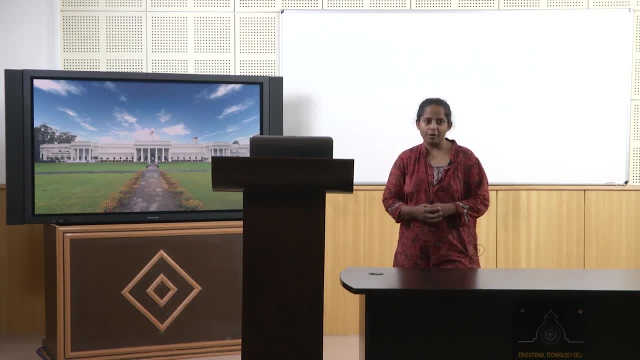 In fact, healthier now because of the immense diversity in your body, But maybe one of them is not good for you And you might fall really sick. So this is external environment impacting internal. Another example would be: I drink water, it has pathogens in it and I fall sick. 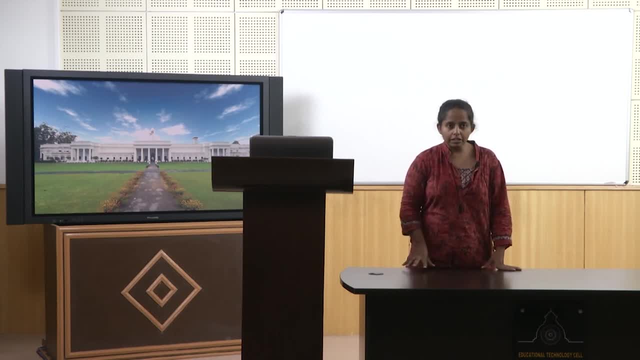 Now let's look at internal impacting the external. One of the major environmental challenges in front of our country today are is antibiotic resistance, And this is a classic example where the internal exchanges antibiotic resistance with the external and external gifts antibiotic resistance to the internal. 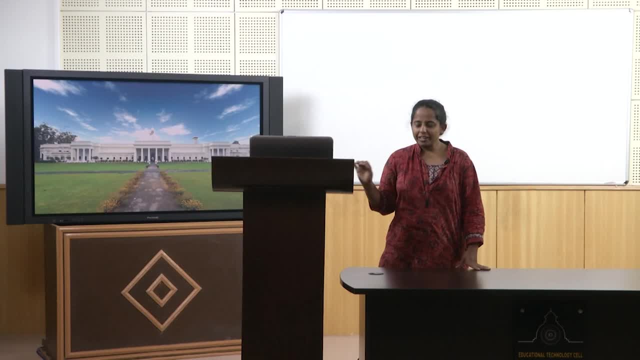 So let's see, So, let's see, So, let's see So in very soon. and this is also the new motto of a leading research department, department of biotechnology- that we have to move towards one health. So environmental health, public health and veterinary health all have to come under one. 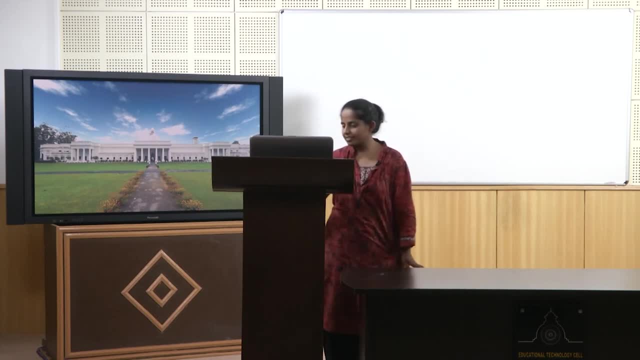 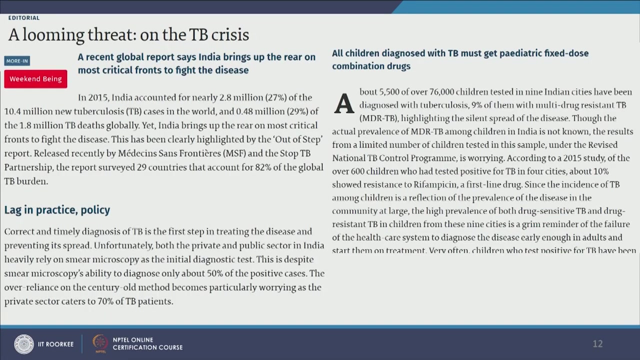 umbrella, because we can no longer distinguish between internal and external. However, in this course, we will be focusing mostly on external environment, And this is a beautiful paper that is pretty recent and we will talk about this paper later, But for now, I think this is enough to know. 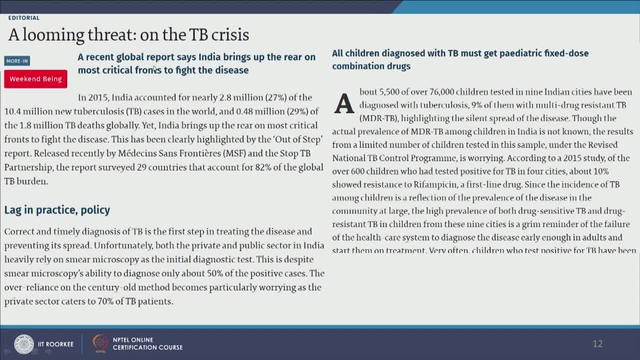 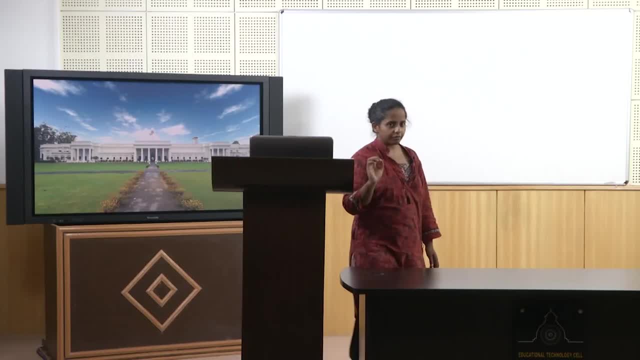 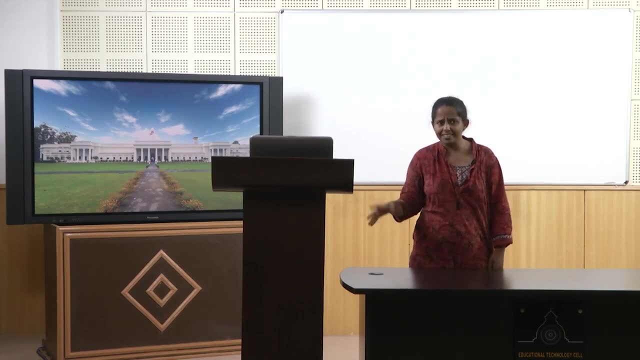 And this is antibiotic resistance threat and I wanted to share this and that how. TB- antibiotic resistant tuberculosis- is a big issue in India And even though it sounds like a very medical problem, well, antibiotic resistant infection- doctors take care of it, medical professionals, medical scientist, biotechnician- but this 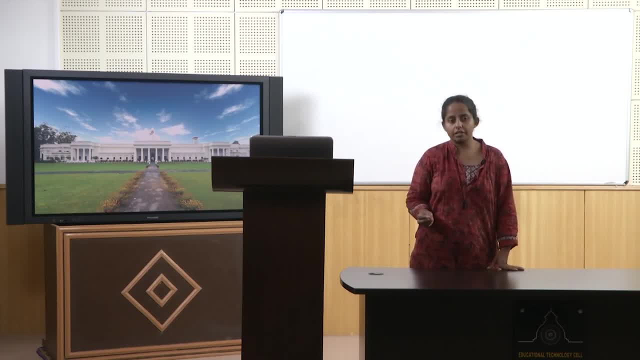 is very important. The latest research suggests that the root cause of resistance in tuberculosis, or any other micro pathogen for that matter, is not what is happening just inside the hospital, just inside the body, and what the dogs are doing to bacteria. but a large role is played. 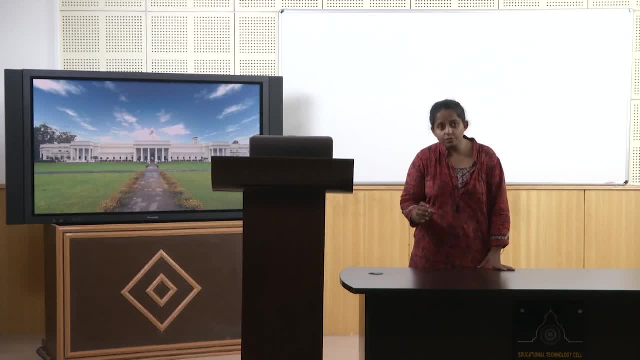 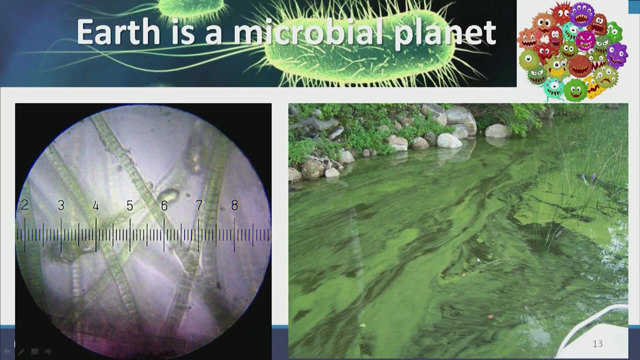 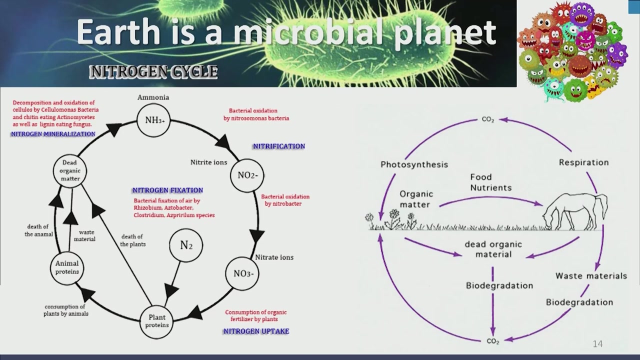 by natural environment, And this is where environmental engineering has to jump into action to help combat antibiotic resistance. All righty, And this is cyanobacteria. by the way, pictures of cyanobacteria under microscope in lake. and remember, This is the bacteria that generated oxygen for the first time on earth. 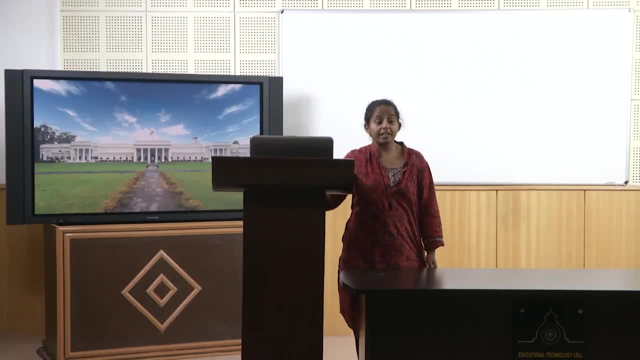 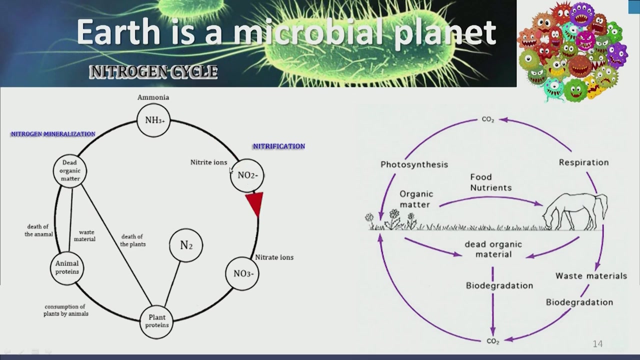 The other important reason why we should spread awareness of applied environmental microbiology is that microbes not only impact health, whether it's environmental, public or veterinary, but they also impact our climate. They impact how our nutrient cycles move on our earth. For example, here we have nitrogen cycle and carbon cycle. both are driven by microbes. 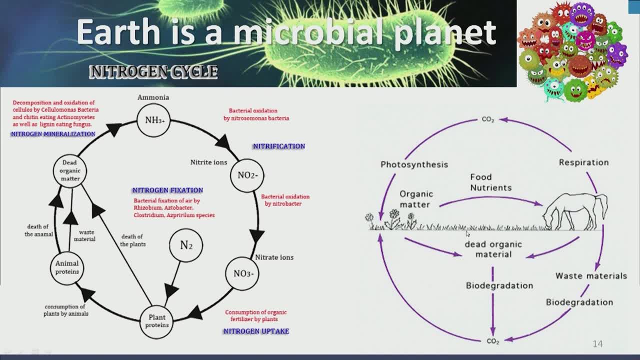 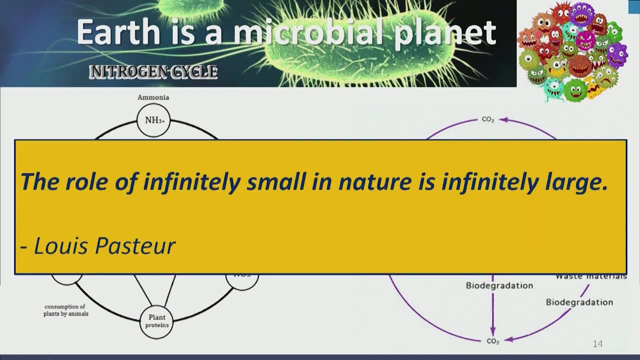 And this is where it becomes very important to understand that, depending on how microbial communities behave, our climate will respond to it, And I would like to quote one of the early heroes of microbiology, Levi Pasteur, that the role of infinitely small in nature is infinitely large. 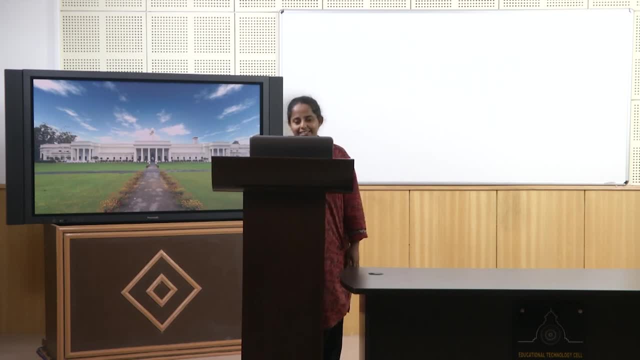 And this is exactly what we are talking about. This is exactly what we tend, we hope, this is exactly the message that I hope to pass on to you, my dear students, in this course. So, because the role of infinitely small in nature is infinitely large, let's understand. 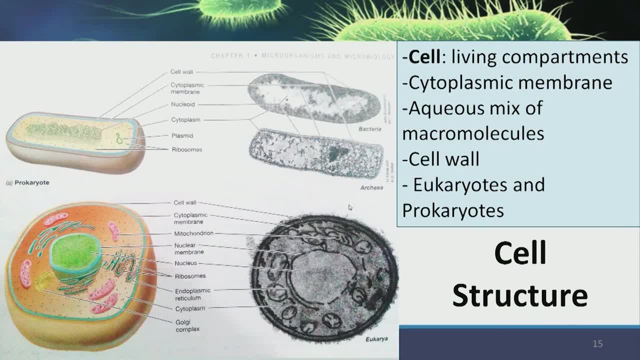 the infinitely small in nature, And we start with the fundamental unit of life: the cell, the cell structure. In this slide you will note that there are two different kinds of cells. On the top we have this very simple container with grey container with the blue inner cell. 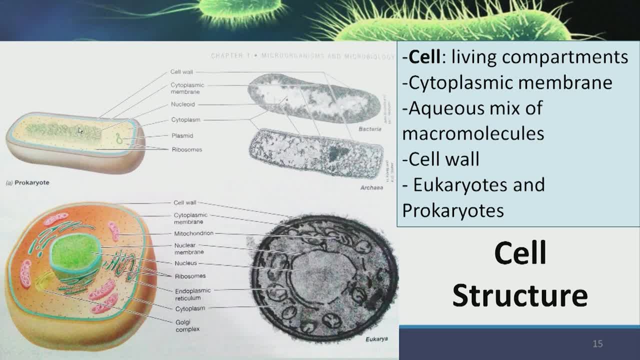 Here with the blue inner lining and some liquid inside and this convoluted green mass. Now let me give it more scientific terms. The layer outside is actually cell wall. The blue layer is cytoplasmic membrane. The orangish liquid here with dots in it is cytoplasm. 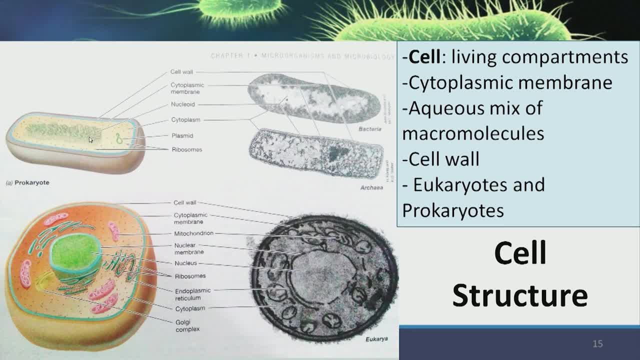 And then this green convoluted mass is actually nucleus. So it is a genetic code. This particular kind of cell is called prokaryote. Pro meaning primitive. Karyote means cell. So this is a primitive cell, not in terms of complexity, again, but in terms of time when 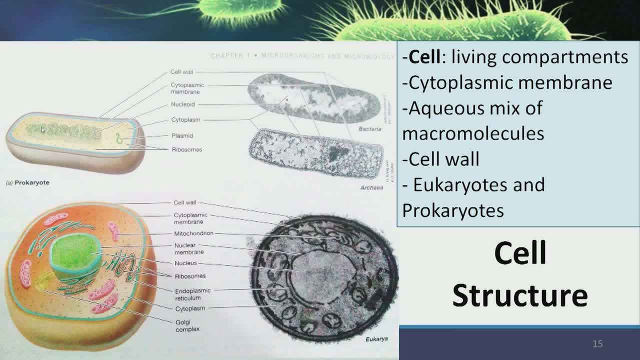 it first evolved. Now it is very important to note that in this cell it has a very simple geometry and it has only one container, So it is like a one room house. In the bottom we have a eukaryotic cell, and I have already mentioned that u means new. 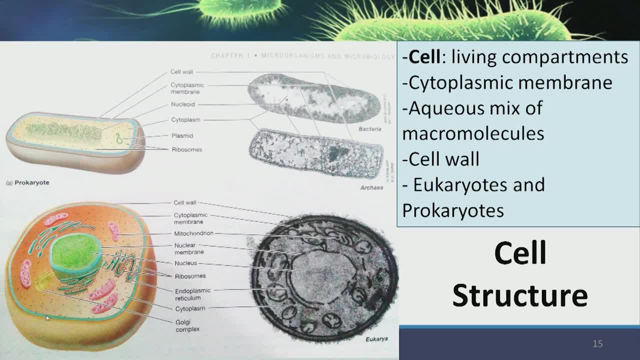 karyon means cell. So in this we have a container, an orange container with a blue inner lining, Some orangish liquid here with dots, and look, there are multiple organelles within this compartment. There is a sphynx mitochondria, there are these blue endoplasmic reticulum and then 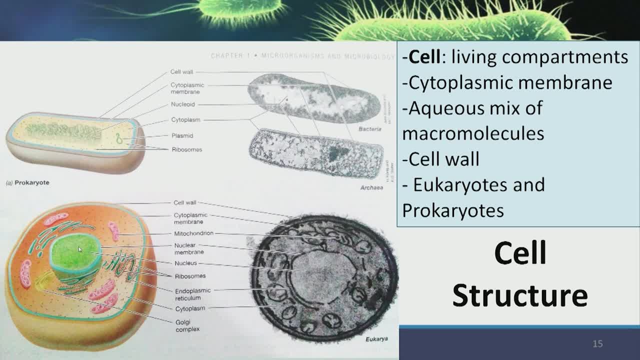 there is this green nucleus with the blue lining around it and the golgi complex is yellow. Now, each of these organs that I mentioned- nucleus, mitochondrion, golgi body and endoplasmic reticulum- They have their own membrane, so this cell in some way behaves like a building with multiple 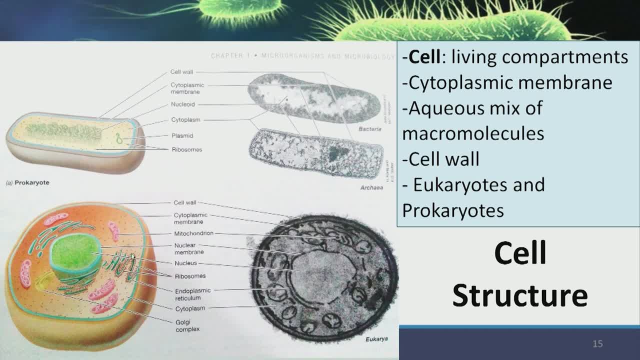 rooms. So if this is a building, it has multiple rooms inside it. On other hand, prokaryote has only one room. it is a one room house. Now, cell is the smallest living independent living being and to enunciate more about the 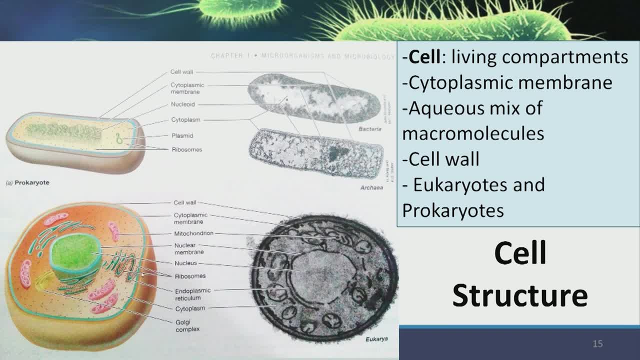 cellular components it is very important to understand. both of them will have cellular membrane and, more often than not, a cell wall. Inside they have cytoplasm. cytoplasm is a water based mixture of macromolecules, biomolecules which are very important. and this is where life happens. the biochemistry of life happens. 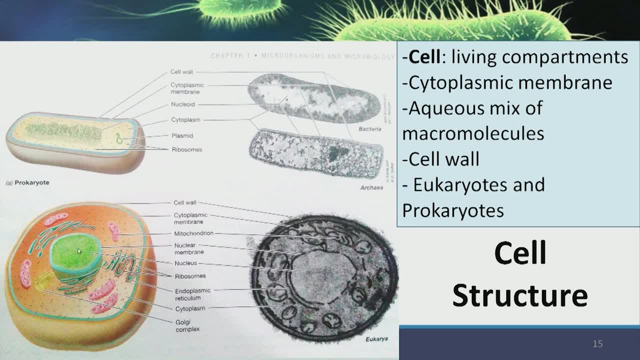 Now this green mass both in prokaryote and eukaryote is nuclear material, which is genetic code. This is the code of life and there are four alphabets in code Code of life: A, T, G, C, and in next lecture we will be talking about A, T, G, C more. 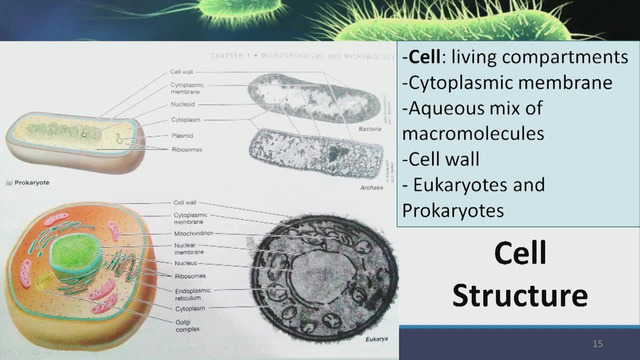 But for now, it is important to understand that the information stored in this green mass is what tells cell how to deal with the day to day activities, the minute to minute challenges and issues that come up. These encode how life will work for this cell. 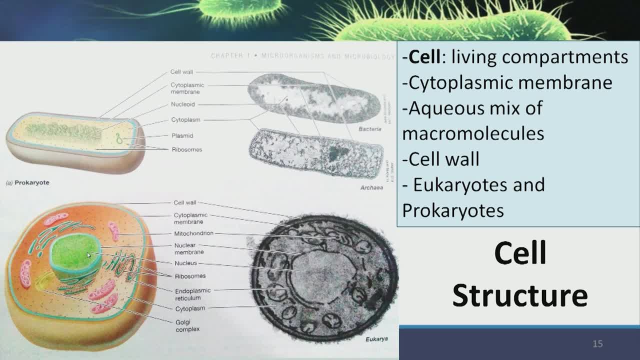 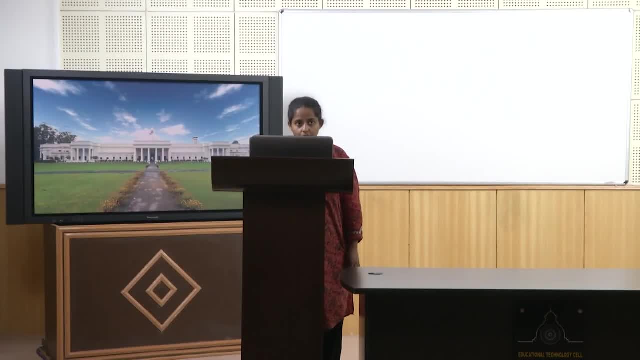 In terms of a eukaryote. let us take our example: our green mass, the DNA, will decide how, what colour are skulls, Skin would be, whether we are going to be humans or not in the first place, How our hair would turn out and what diseases we are susceptible to. 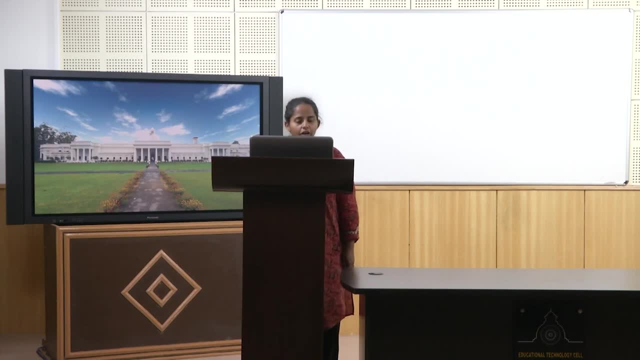 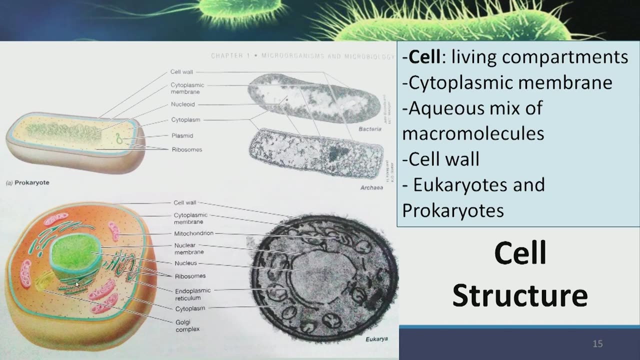 I want to mention that these two pictures on the left for prokaryotic and eukaryotic cell are artistic impressions. These bodies do not really have these colours but they are helpful to visualise in a class. On the right side we have more real, microscopic images of two prokaryotes and one eukaryote. 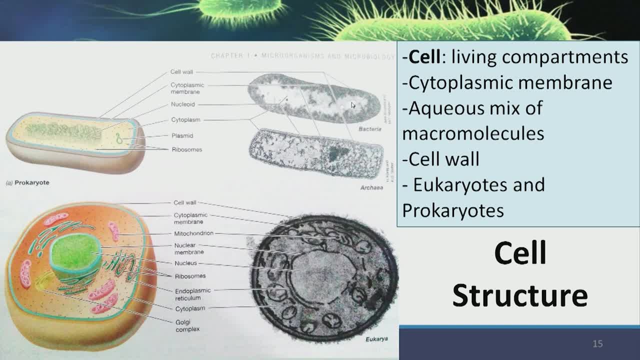 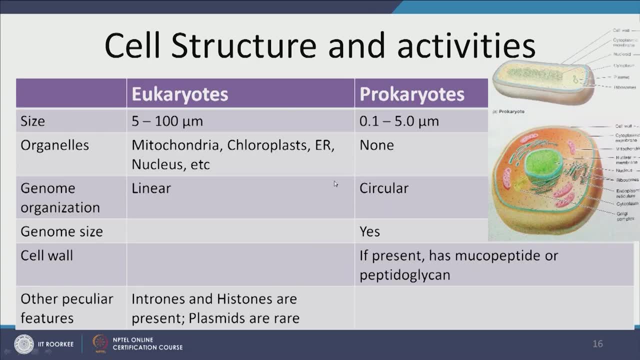 And the good question that I want you to think about is: why do we have two prokaryotic examples and one eukaryotic example? We will talk about it in next lecture, But for now, I think it is important to know that eukaryotic and prokaryotic cells are. 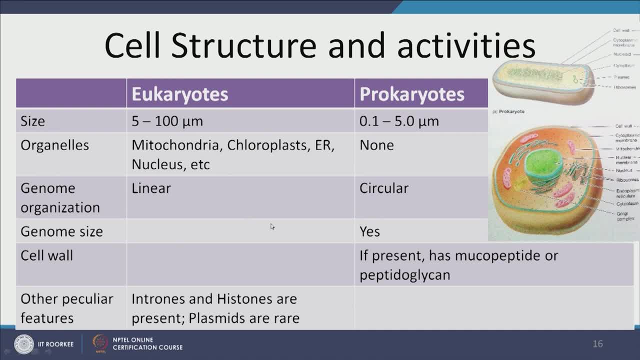 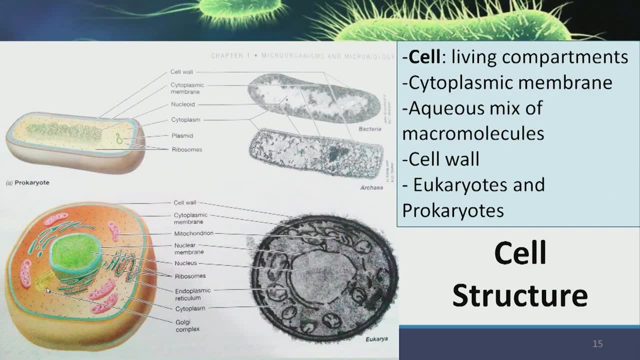 different from each other And I will go over these details, these in detail, later. So for now, it is just important to know that the pro eukaryotic cell is much bigger than prokaryotic cell. Eukaryotic cell has multiple organelles with separate individual organelles. 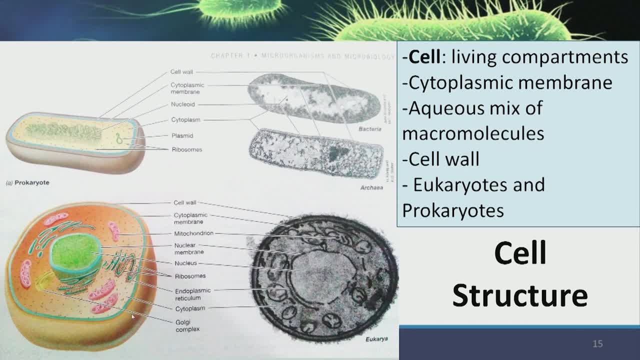 So for now, we will talk about that, Thank you. So eukaryotic cell has multiple organelles with separate individual membranes, whereas prokaryote does not. The nuclear material in eukaryote or genetic material in eukaryote is much longer and much. 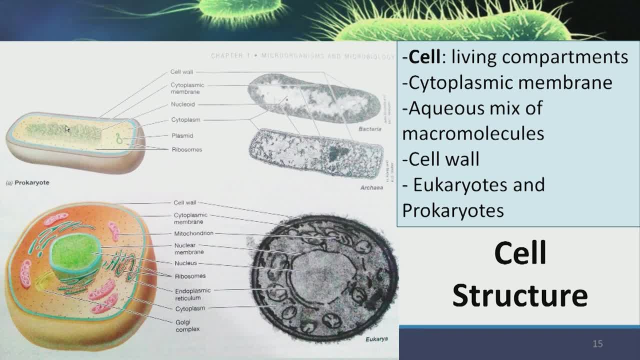 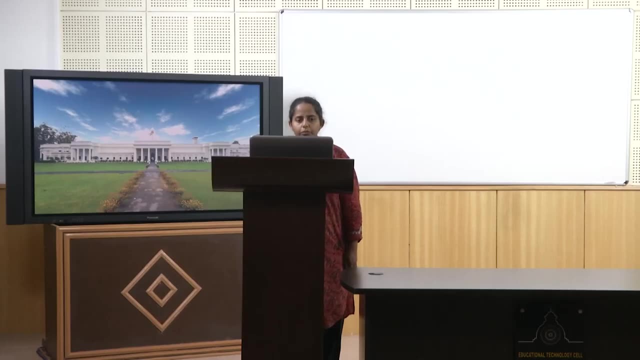 more complex than one in prokaryote. Eukaryotic nuclear material also have very interesting things like histones and do not have plasmids that are very often found in prokaryotic cells. Another important difference in between prokaryotic 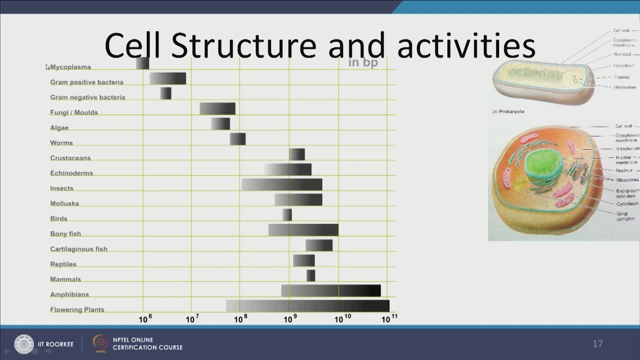 and eukaryotic cell is the off size. Most prokaryotic cells- here the examples are microplasma, gram positive and gram negative bacteria are less than 10 to power 7 base pair per cell. Most eukaryotes are much larger and that is the reason why it is. it was so easy and so 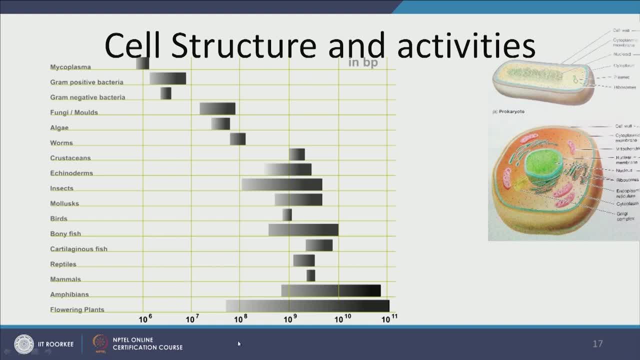 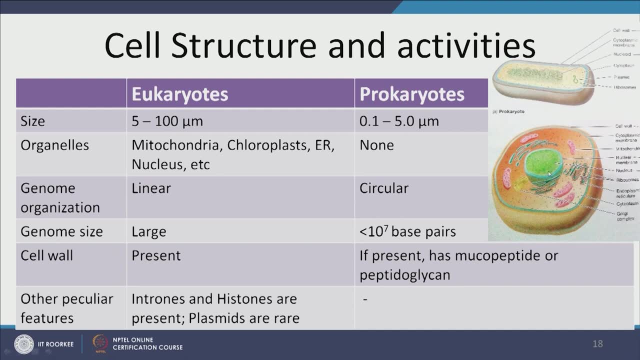 convenient to sequence the bacteria much before we could manage human genome. In fact, it is interesting to note that in case of prokaryotes, which are bacteria- which bacteria is an example of prokaryote, by the way- In case of bacteria, an individual lab could sequence the entire genome, but for human, for. 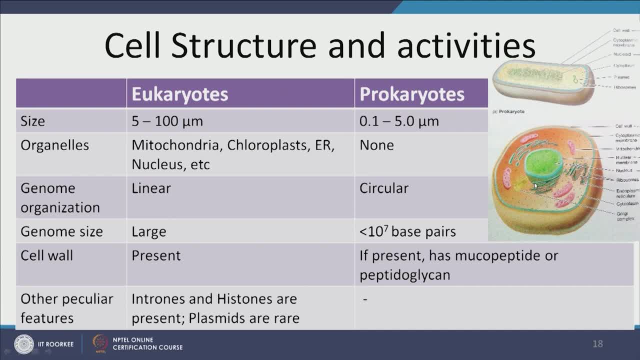 many years we had to rely on a massive human genome project. And then the other difference between eukaryote and prokaryote would be: the eukaryotic genetic material is linear, whereas for prokaryote it is circular. So if we could unwind. 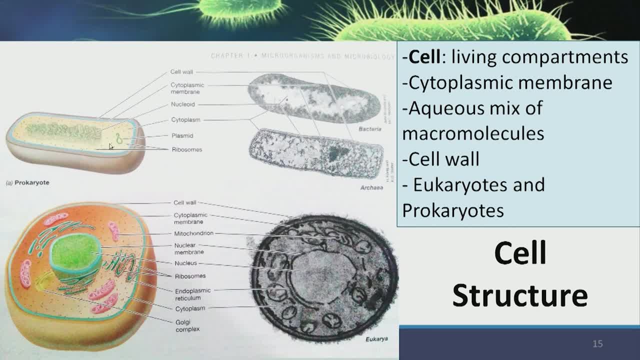 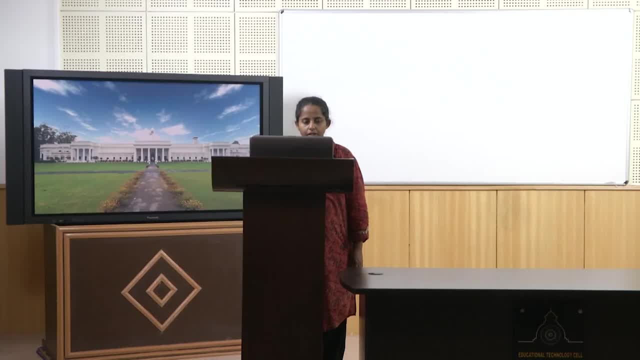 If we could unwind this green convoluted mass here. So if we could unwind, If we could unwind this green convoluted mass here, for a prokaryotic cell it will come out to be a perfect circle, and for eukaryotic it will come out to be a straight line. alrighty, 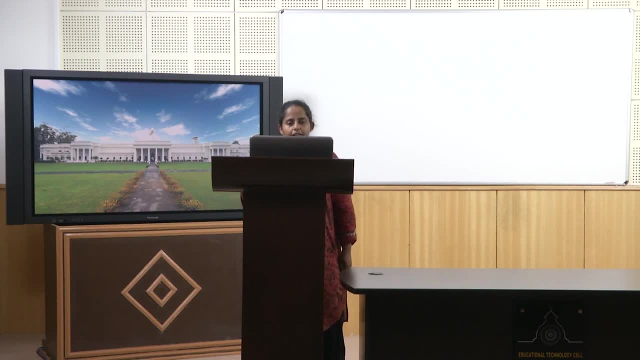 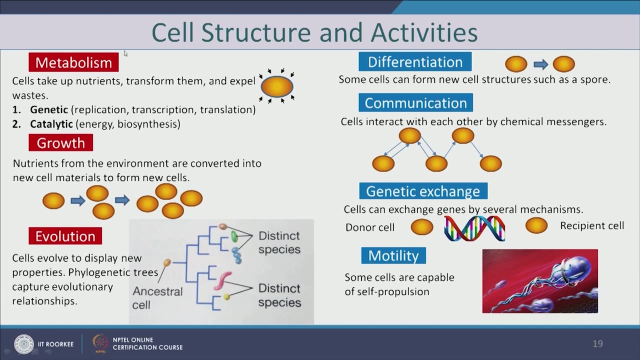 Now, what does a cell do and what its structure is Now? on left side, we have important activities of the cell, such as metabolism, growth and evolution- that it does on its own, individual level. On right side, we have differentiation, communication, genetic exchange and motility. this is how. 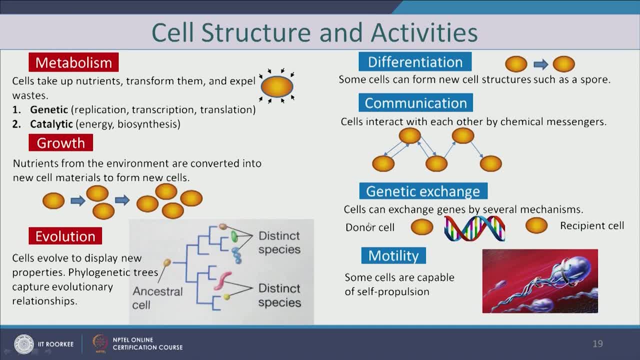 a cell behaves, Interacts with its environment and its colleagues. So let us look at metabolism. cells take up nutrients, they transform them and expel the waste, much like what higher orders of life do. And in terms of metabolism, it has two components: genetic and catalytic. 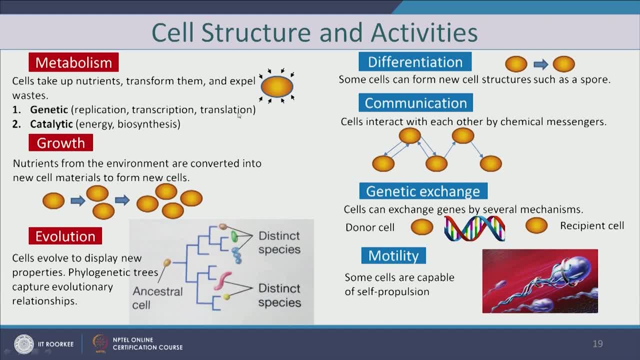 Now, genetic activities would include replication, transcription, translation. we will go over them in next class in much detail. so for now it is just important to know that when it comes to cell activities, It has two components: genetic and catalytic, which is basically genetic and chemical. 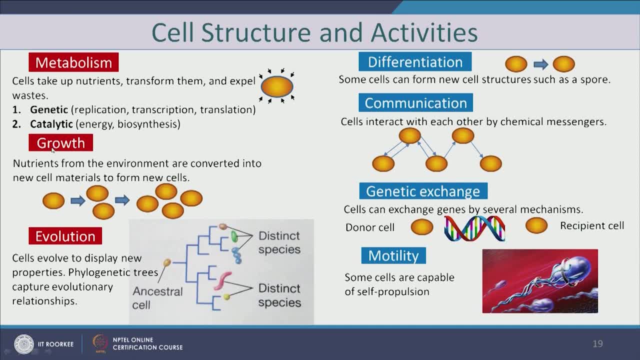 The other important activity for cell is to grow right. a cell needs to multiply, it needs to grow, So from one cell it needs to gather enough material, enough energy and enough nutrients that it can divide into two daughter cells, and so on and so forth. 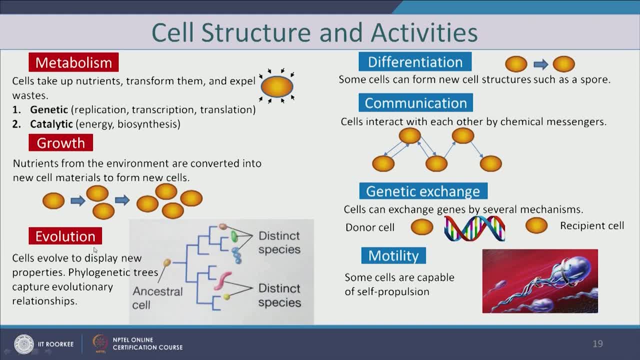 The other activity that cells participate in is evolution. cells evolve at every step of reproduction. So here we have one cell and shoulder one. so here we have one cell and it splits into two daughter cells. right here, in between this replication process, There is a possibility that the cell, the daughter cells, will be slightly different from the. 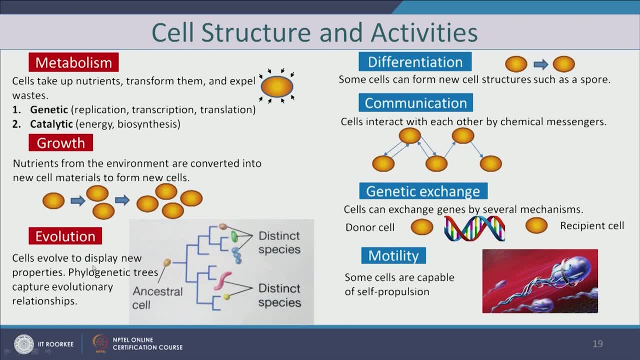 parent cell, and the reason for that is evolution, that genes within the microbes, their genetic material, evolve, change And as such we might have one ancestral cell and it will create many progenies, which the progenies might go and cluster. 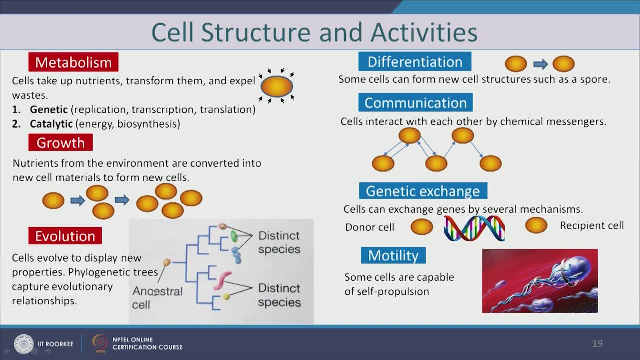 and cluster into unique species and from one ancestral cell we might have very distinct species that look different, behave different and are genetically very diverse, And in fact there is a belief in biological community that we all have one common ancestor, LUCA, and we will talk about it in the next lecture. 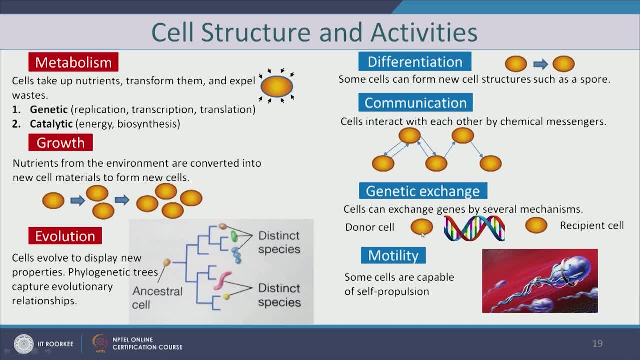 Then we have, on the right, we have differentiation, communication, genetic exchange and motility, and I like to just quickly summarize here that differentiation is when a cell can transform into something else. So we have a living, vibrant cell, but conditions around it go really bad and it decides to. 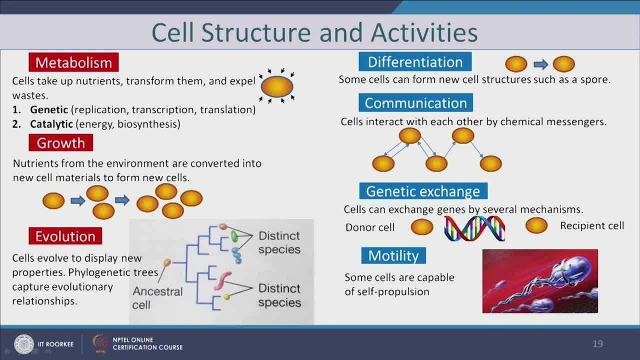 become a spore, So this is different from growth. please keep this in mind. Then we have communication. much like human beings, cells also communicate with each other. They produce these beautiful chemicals which act like messengers, and anyone who catches the chemical and knows how to decode it will know what the message is and our science suggests. 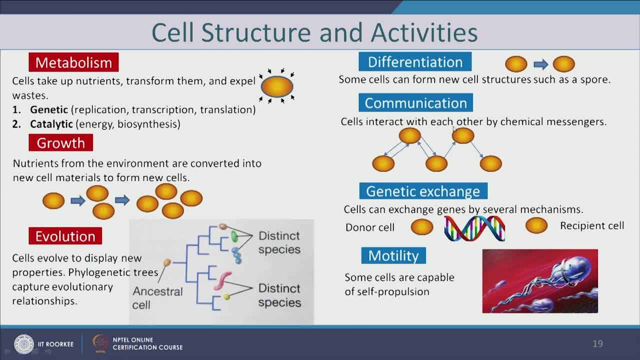 that antibiotics are produced by bacteria to talk to each other, And to this end we have a lot of unfamiliar, unfriendly microbes. The other thing cells do is genetic exchange. This is really cool. a cell can share its genetic material with another cell just by. 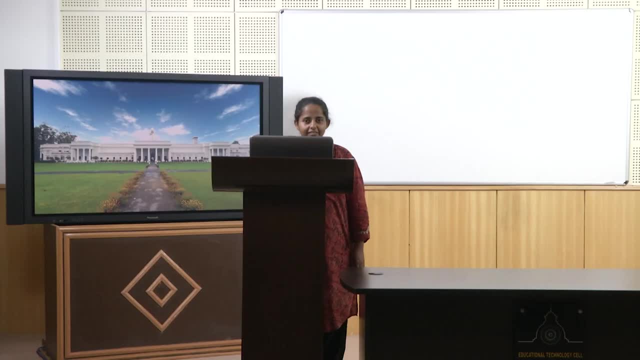 touching. This is almost like saying, if I have curly hair and I touch my friend who has straight hair, I can give her genes to have straight hair, cool, right. And this is also a reason why we have lot of environmental challenges. so this is very 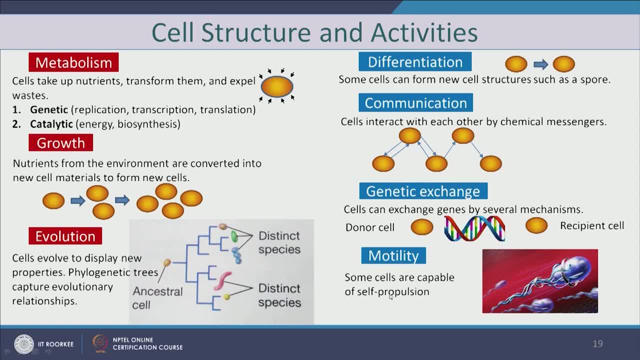 relevant. And next important thing is motility. Cells have capacity. Some cells- not all- have capacity to propel them, and in this picture you have this beautiful microbe with lot of appendages here. What they do is they twist in a particular direction and they act like a supercoiled. 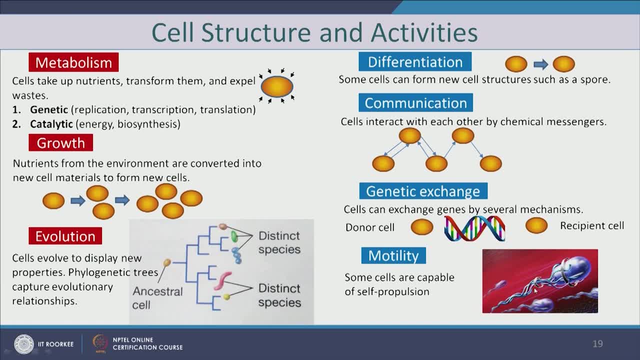 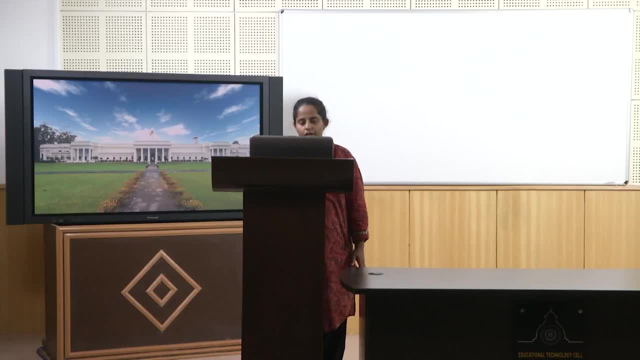 spring. So the moment the bacteria decides that I am ready to move forward, it will let the spring uncoil and it is propelled forward. When it wants to change direction, it just ask its flagellum to. no, it does not ask it just. 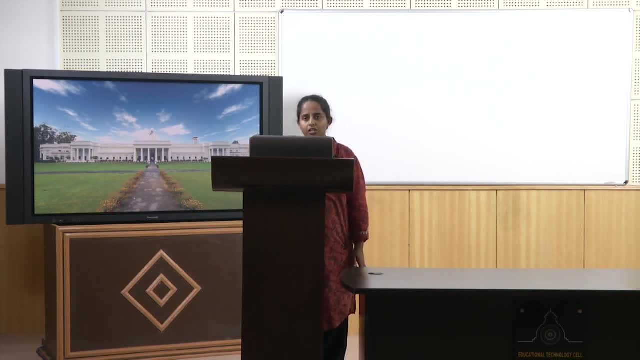 whips its flagellum in opposite direction and it comes to a standstill. And then it can come to a standstill, And then it can come to a standstill, And then it can coil in a different direction to oppose it to which it wants to go.